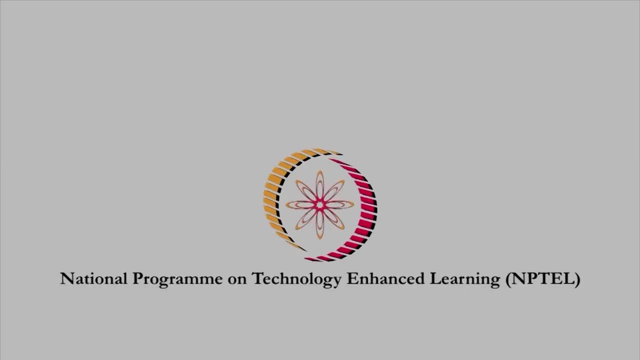 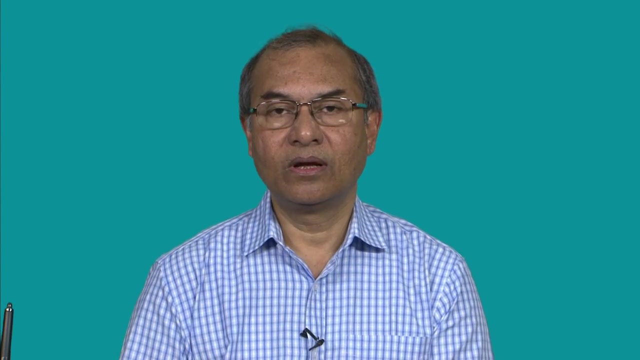 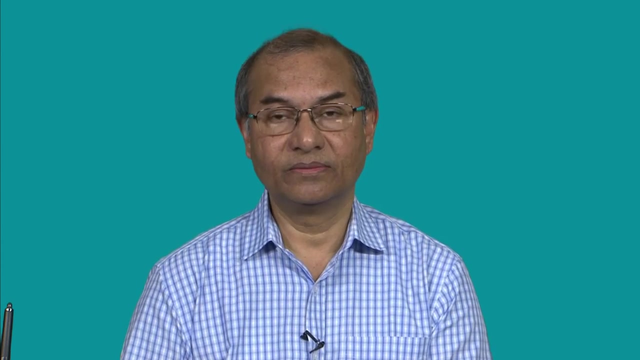 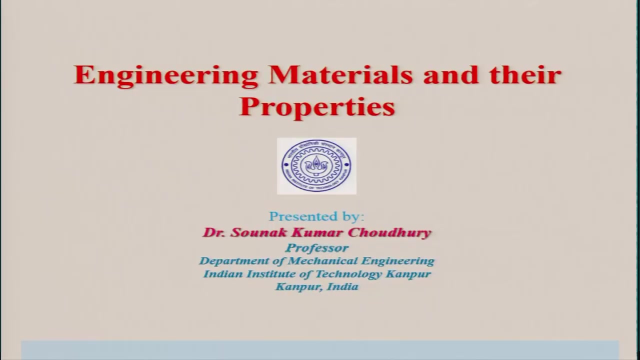 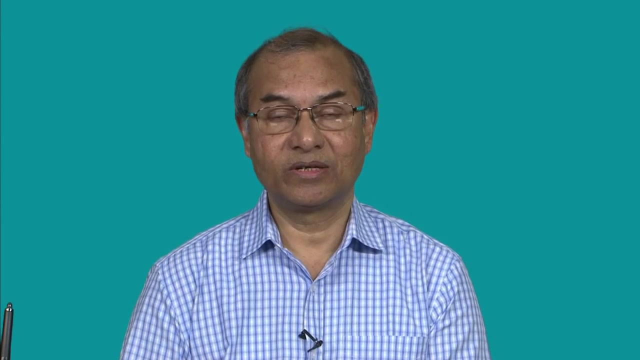 Hello and welcome to the discussion series on the production technology theory and practice. My name is Dr Sounak Kumar Choudhury. I am a professor in the mechanical engineering department of IIT Kanpur, teaching here for the last 34 years. My specialization is manufacturing. 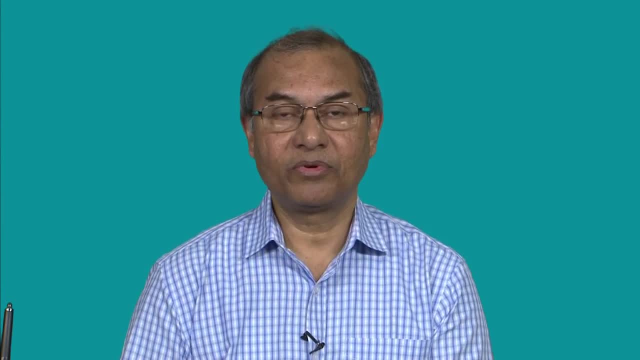 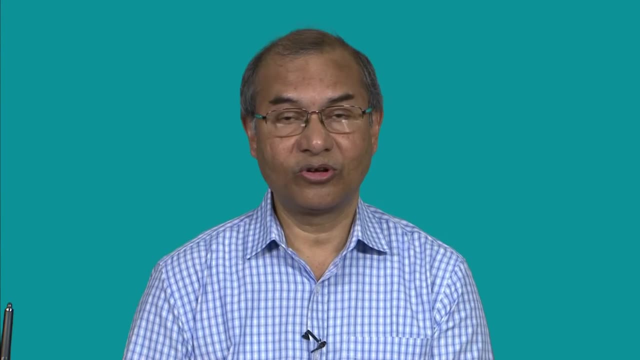 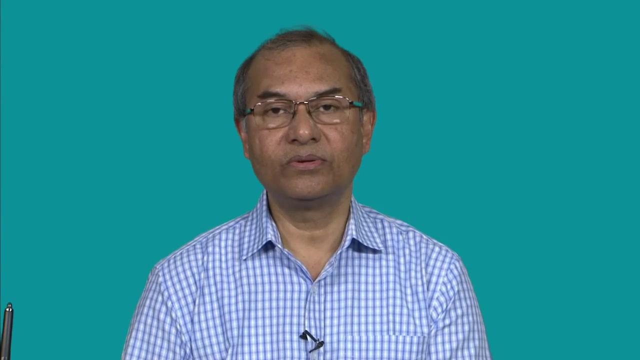 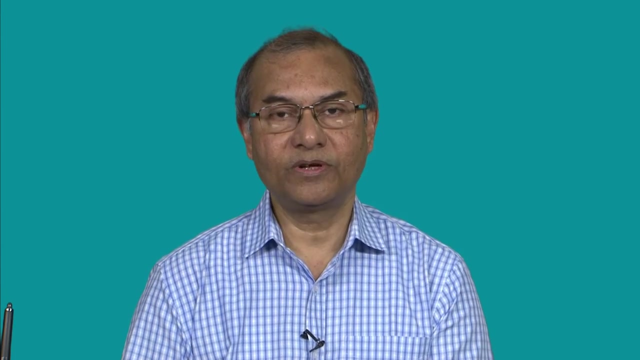 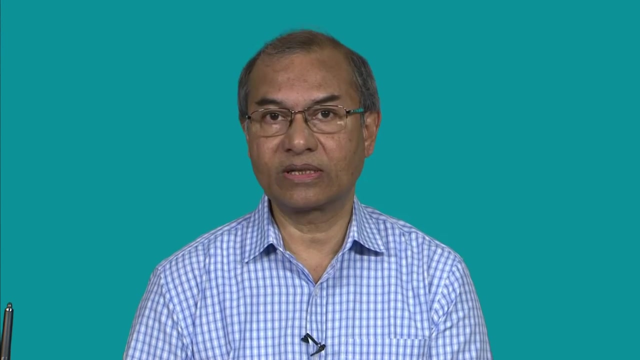 science in mechanical engineering. Apart from that I also work on the unconventional machining, NC machines. So in this series of discussions we will have five modules apart from the lab. So the first module is the materials: engineering materials and their properties we will discuss 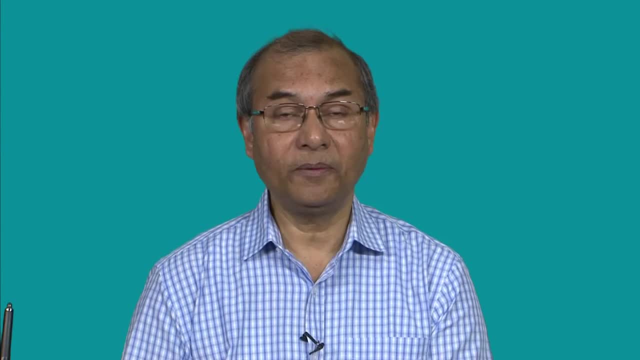 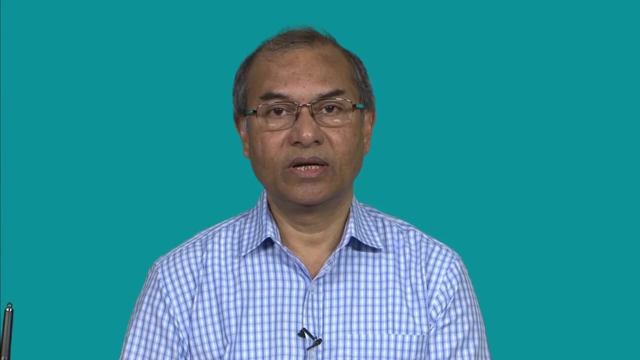 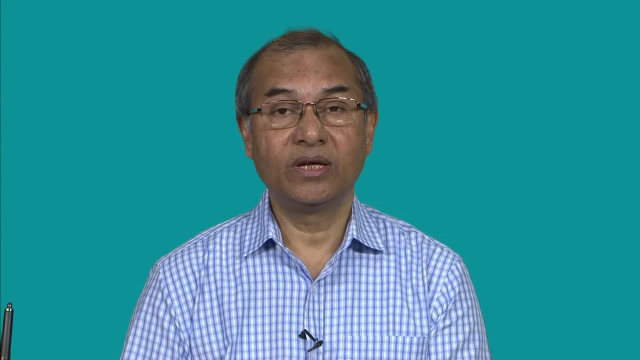 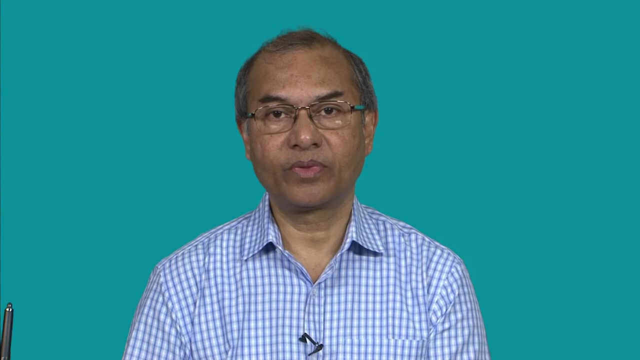 Next module will be on machining, On the conventional machining. So there we will discuss the theoretical background on the machining processes. We will look into various practical machining aspects. We will see how the some of the very simple simulations or mathematical models are built up. We will see the thermal aspect. 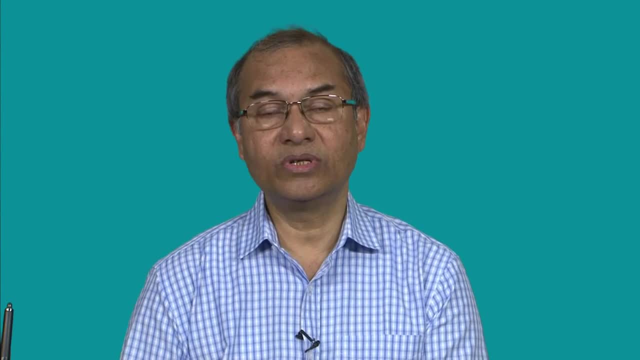 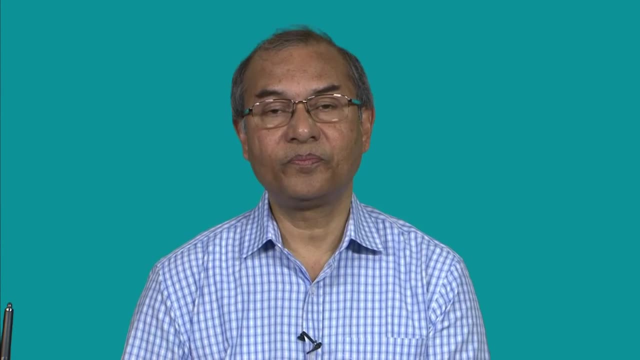 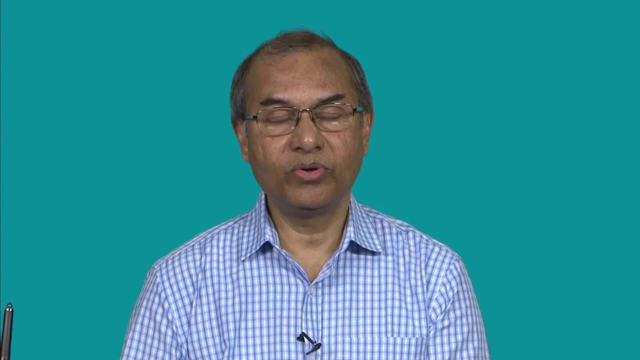 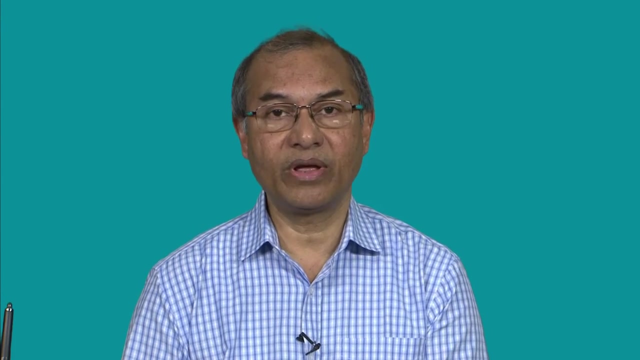 of machining, Stress, strain, how the chips are removed, What is the tool, How the tool wears out, And so on. So there are different aspects. Basically, many things are known to you, But we will discuss the reasoning, mostly that why things happen that way, For example, why 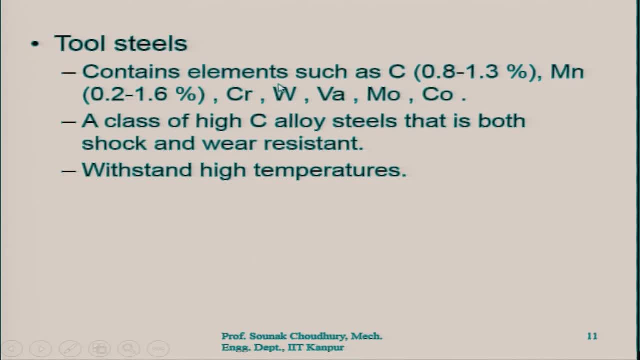 Wolfram. so this is the tungsten. Now, as you again understand, I will just repeat once more that this is the range. so, depending on the exact carbon content and depending on the exact manganese percentage, for example, you can have different properties in the tool steels, so tool steels grades can be different. 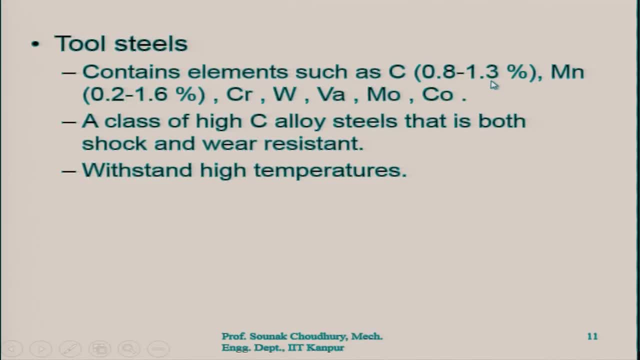 depending on the percentage of carbon within 0.8 and 1.3 percent, The percentage of manganese within 0.2 to 1.6 percent, and so on. Now these percentages of chromium, tungsten, vanadium, molybdenum and the cobalt, these 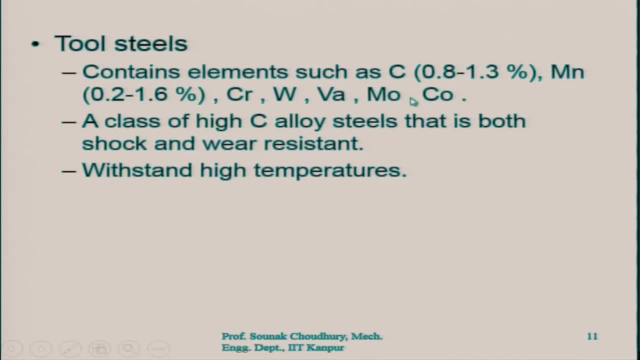 percentages are very small, so therefore they are not really mentioned. it it is about, for example, in some of them it is 1 percent, some of them- well, 1 percent is higher, rather, because it is almost comparable with this. in some places it is about 0.6 percent, and so on. 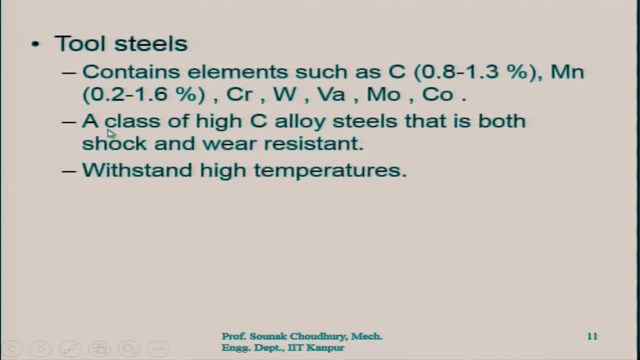 Now the other properties are the class of high carbon alloy steels, that is, both shock and the wear resistant, Now tool steels. this is, you know, it is a modification, that is a another class of the high carbon steel alloy steel and it has both shock and the wear resistant. it can withstand the shock. 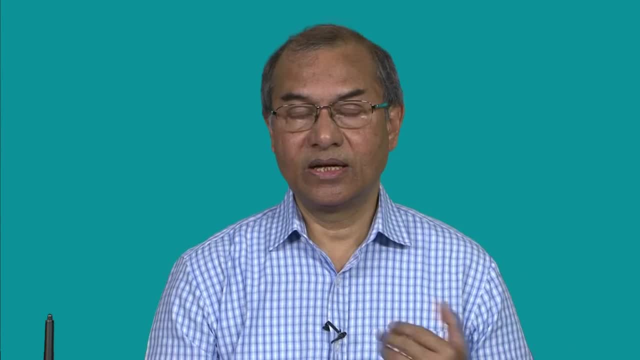 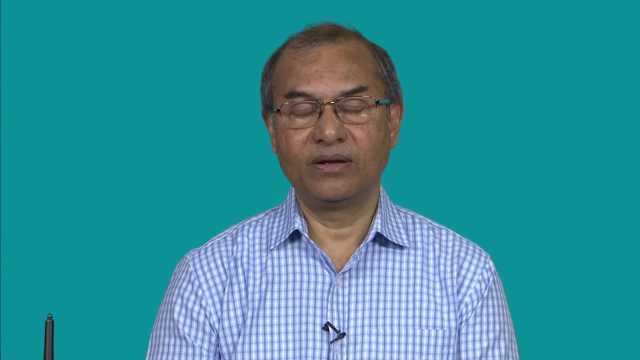 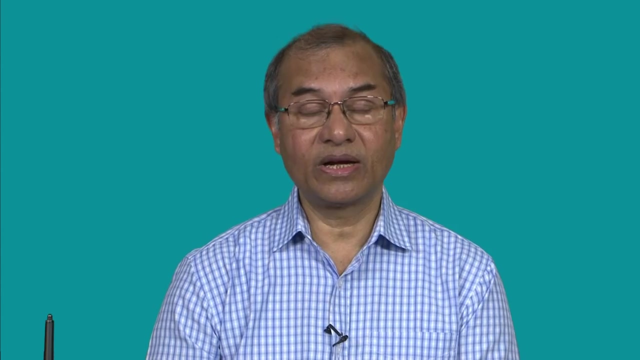 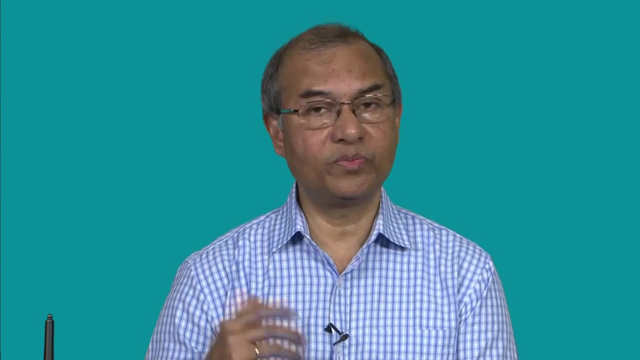 Now where we need that shock resistant: in the tool steel. Now it is. You understand that when the say if we have a turning tool, the single point cutting tool, and it is used, it is fabricated out of the tool steel. So in case of inhomogeneous hardness in the workpiece which may happen because of the 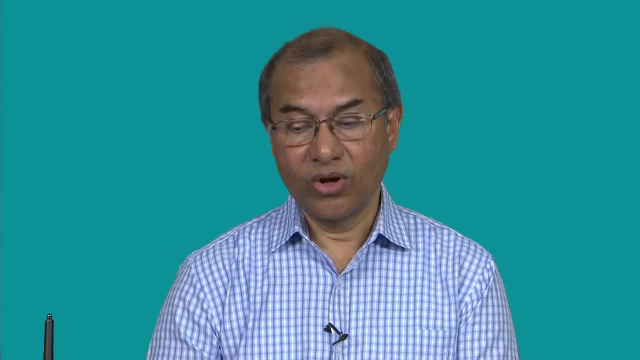 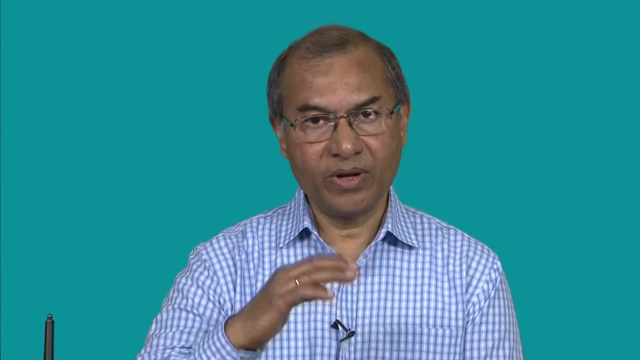 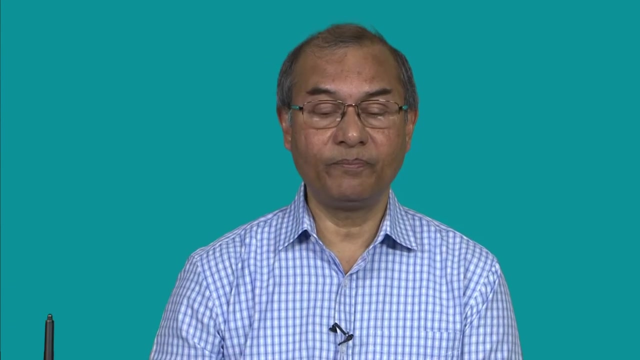 hard particles, inclusion inside the workpiece. so whenever the tool is cutting, going through the material And because of the inhomogeneous hardness, there will be different kind of work. I mean the forces will fluctuate. So because of that fluctuation there will be some shock to the tool. 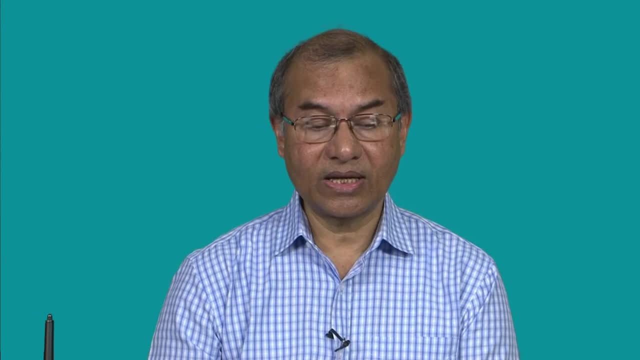 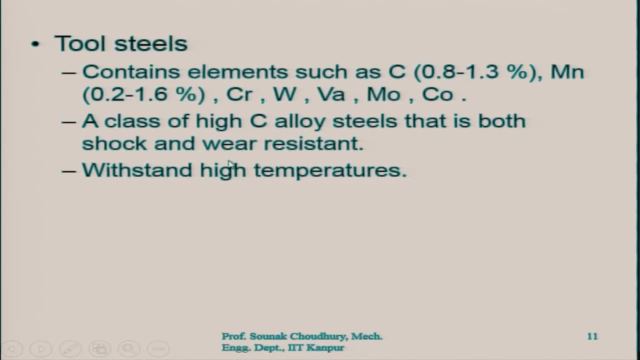 So that has to be withstood. and this kind of tool steels, which is another class of the high carbon alloy steel, as it is written. as I told you, It has this property. So this is the shock resistant As well, as it can actually resist, where, to a large extent, 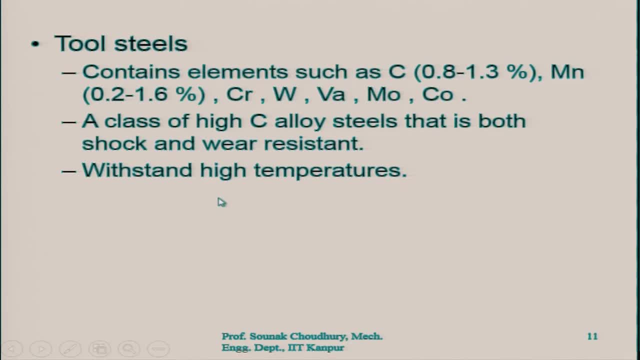 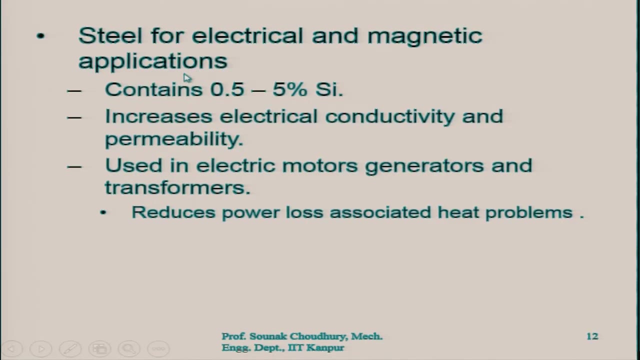 Ok, Withstand high temperatures And withstand high temperatures, particularly that it retains its hardness with the elevated temperature. At an elevated temperature, higher temperature Steel for electrical and magnetic applications. So those compositions will be different because the demands of from those steels in the area. 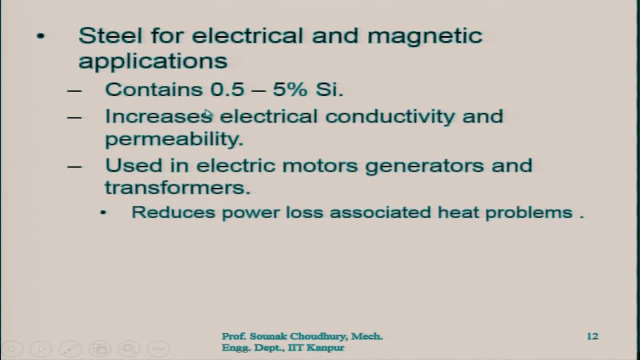 of electrical And the applications will be different. Now those kind of steels you are may have the 0.5 to 5 percent of silicon that increases the electrical conductivity because we need it for electrical usage, application and permeability. So because of that these two conduct, these two properties, that the conductivity and permeability. 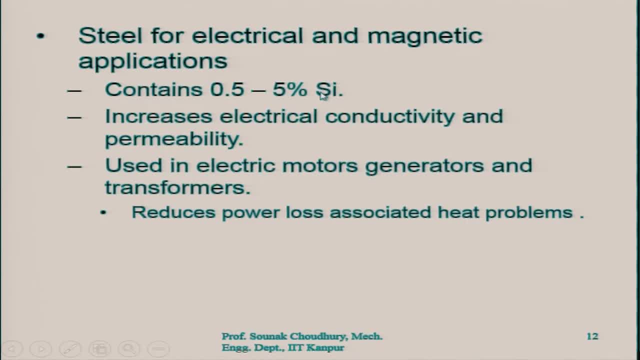 the, which is which is which is given by the silicon. So percentage can be varied from 0.5 to 5 percent. depending on, again, exact percentage of silicon, you will have the different grades and levels of the permeability or the electrical conductivity. Such kind of steels are used in electrical motor generators, for example, when the you. 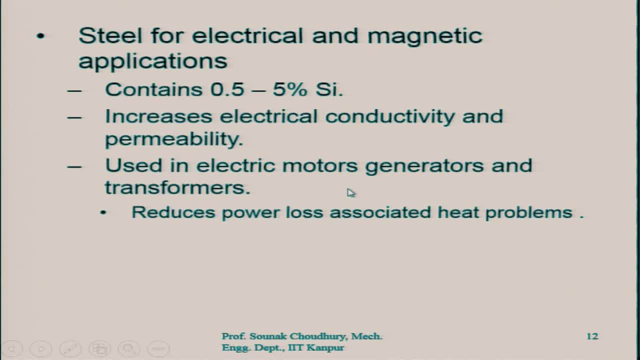 know the binding, the wire which is required for making the bindings, and the transformers in transformers, and the motors, apart from the housing, apart from the structure and the wire that is required, all these you know. material can be this kind of materials, with the silicon percentage up to 5 percent reduces power loss associated. 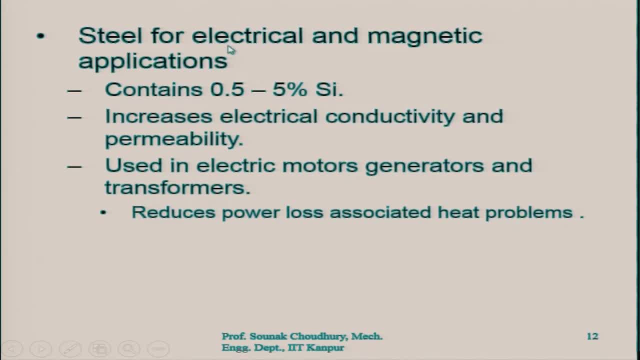 with the heat problems, Meaning that. So these steels are specially made so that at high current and the high voltage, the temperature which is produced there, the power loss should not be there In the case of transmission- this very important thing- and so that the output could be according. 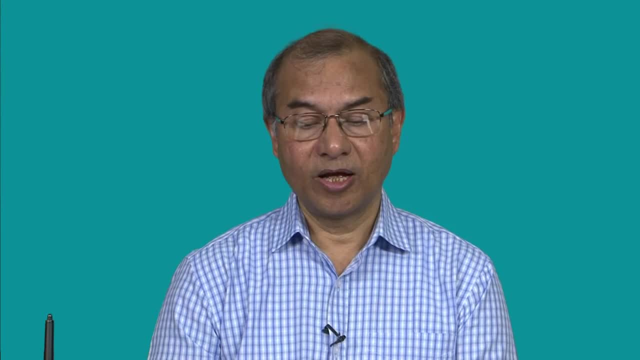 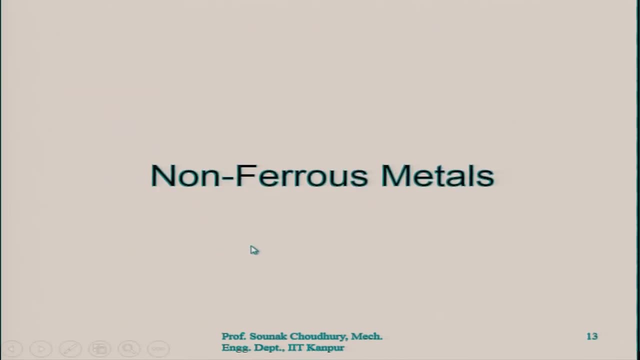 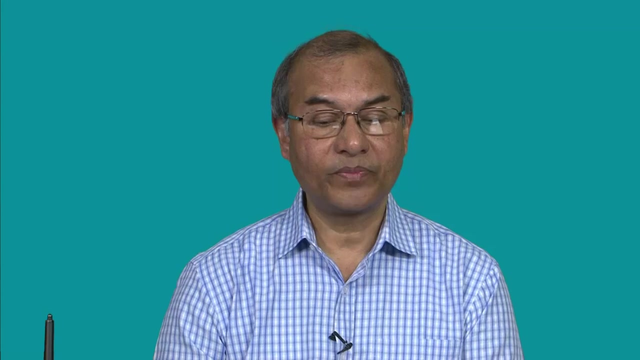 to the input that is given in the generators or the motors and transformers. Let us discuss some of the non-ferrous metals. 1. non-ferrous metals and let us see how they differ from the ferrous materials in terms of properties, in terms of usage and so on. 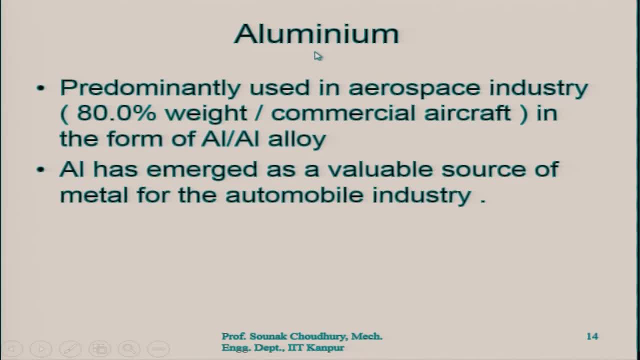 Let us say first, representative of the non-ferrous material is, of course, aluminum, which is very widely used and, as you understand that this is a light material, this is a cheaper, relatively cheaper material. of course, it is not so cheaper than not as cheap, as I mean not cheaper than. 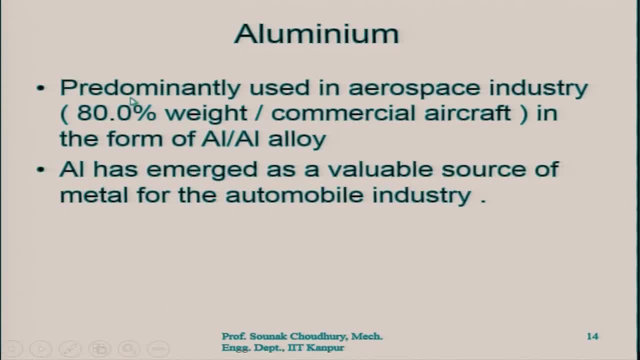 the steel and so on, But nevertheless it aluminum predominantly used in the aerospace industry because it is light, as I said, and 80% weight by commercial aircraft. in the commercial aircraft this is borne by the aluminum parts, the parts made of aluminum, Aluminum and the alloys. of course it is not pure aluminum, as you understand the entire. 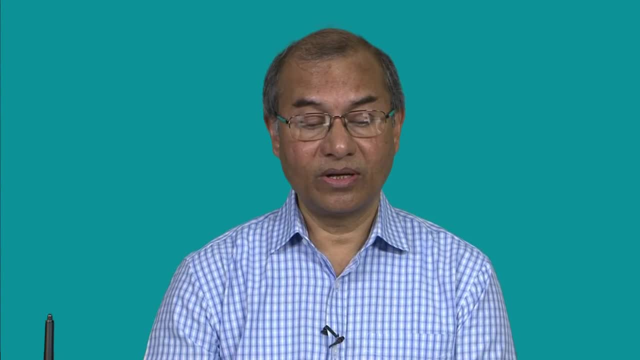 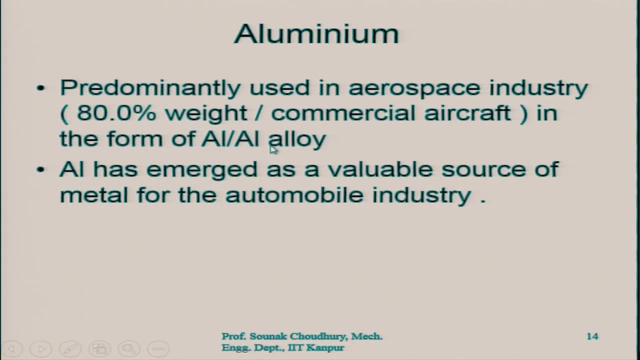 housing, for example. okay, And so on. this is in the form of aluminum or aluminum alloy, with I am coming to that aluminum alloy, which will give you different properties of the aluminum. Aluminum has emerged as a valuable source of metal for the automobile industry again. 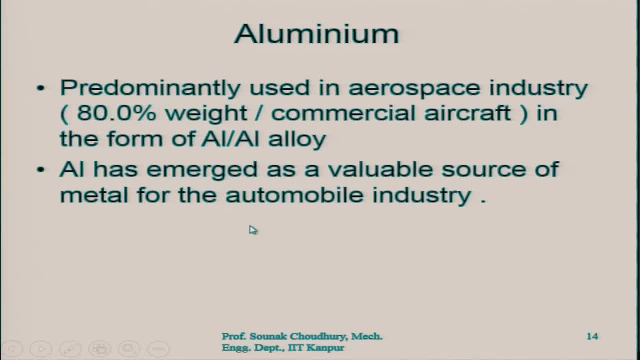 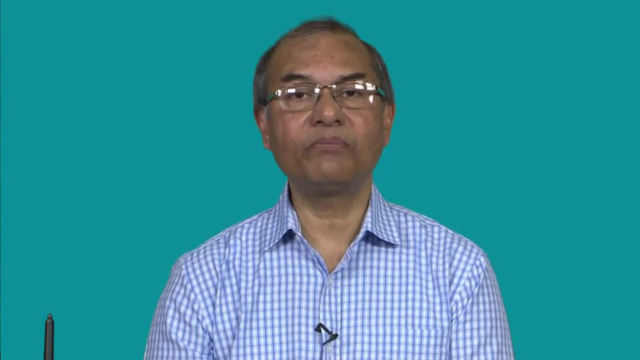 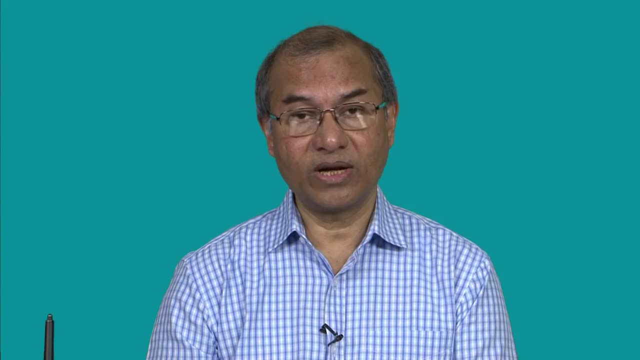 because of the light weight, because of the sufficient strength. okay, Of course, it is again the aluminum alloy, mostly not the pure aluminum, And because of these properties, the in the automobile industry it is very popular, as you understand, and basic thing is that when the automobile is becoming lighter it will. 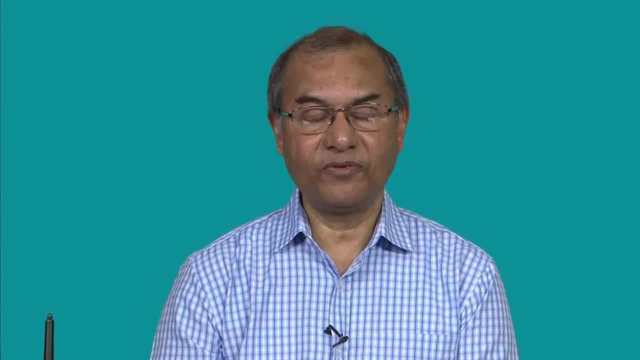 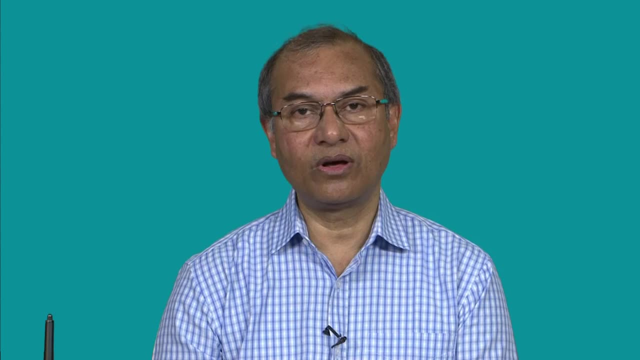 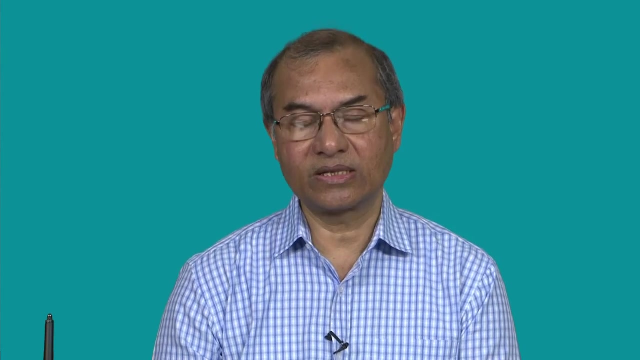 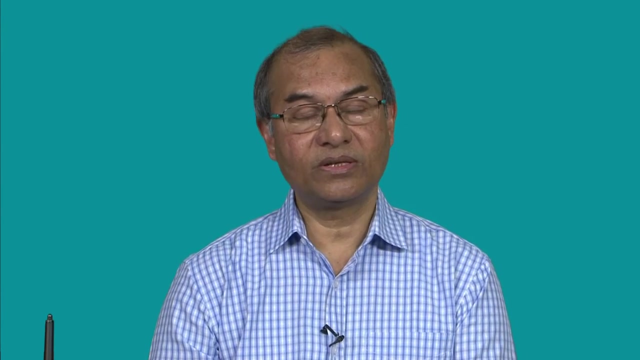 actually consume less power. So therefore, it will consume less fuel, and that is very important. and if we are gaining weight, I mean gaining in the weight of the automobile. this is a drastic reduction in the power and drastic reduction in the fuel. Okay, So fuel consumption can be achieved, which actually are being such automobiles are being 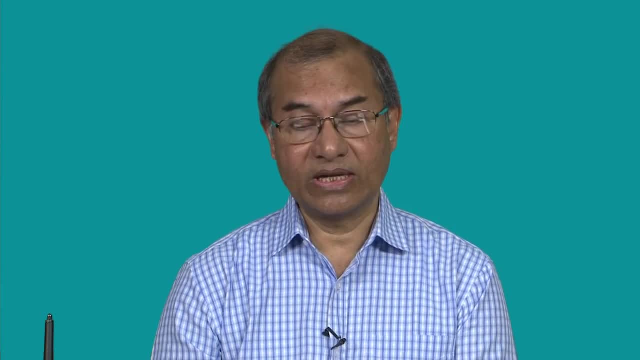 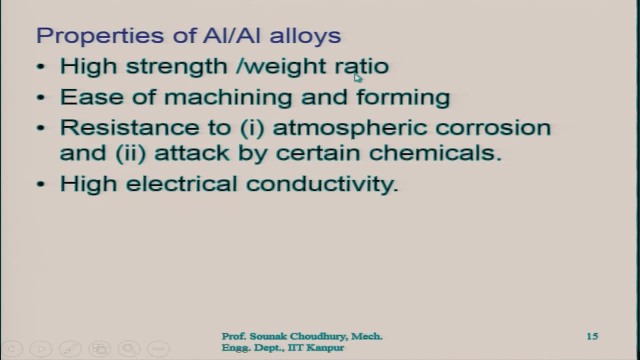 designed these days and which you can see on the roads these days: Properties of aluminum and aluminum alloy. So high strength to weight ratio. okay, the ratio of the strength to weight is very high. So you understand that for less weight with very high strength can be achieved. 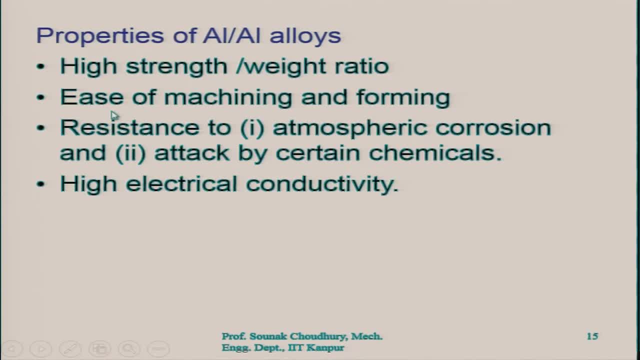 So therefore, that strength to weight ratio can be very high. Okay, Thank you. Ease of machining and forming because it is relatively softer material, okay. So therefore the machinability is good and for formability is better. So using the metal forming you can have the different kind of different kind of parts. 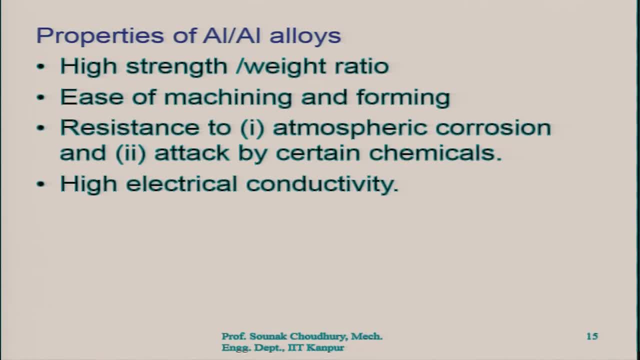 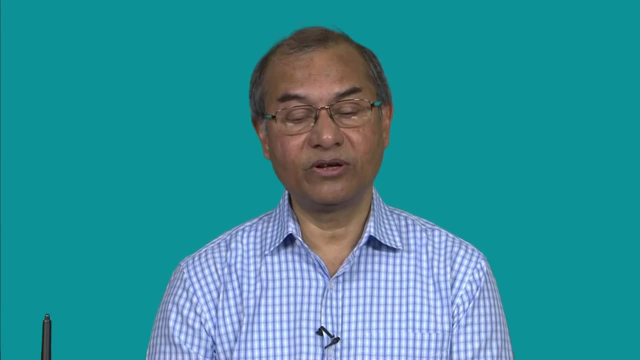 using the casting, as you understand, of the aluminum, you can have different kind of parts. So after casting it can be actually machined easily If it is required. similarly, after forming it can be given a finish shape if it is required. So that case machinability of the aluminum will be better and it is very desired property. 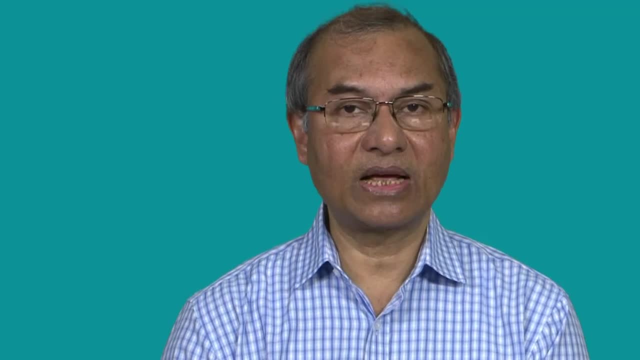 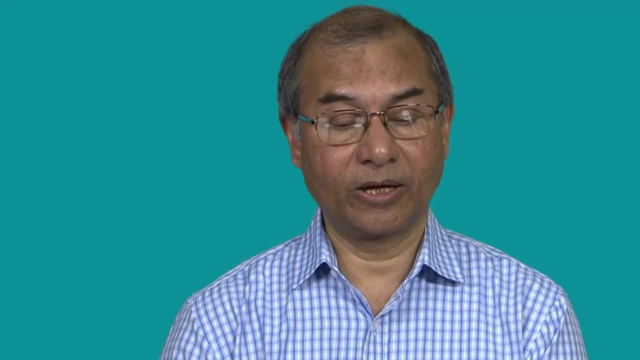 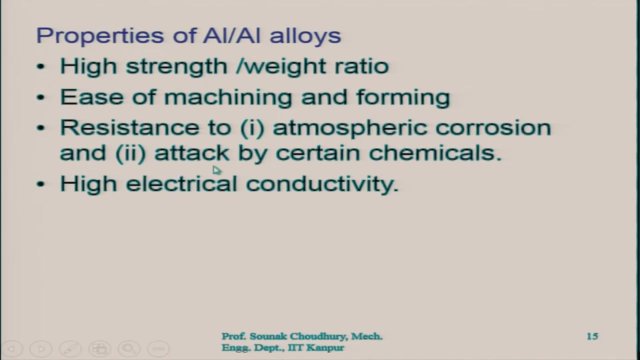 because, in many cases, after the casting, after the metal forming out of aluminum material, we need to have the final shape by machining. Next property is the resistance to atmospheric corrosion. Okay, Okay. So what is the resistance? It is to attack by certain chemicals. 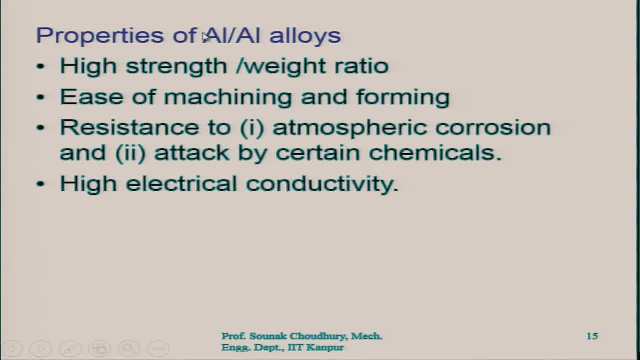 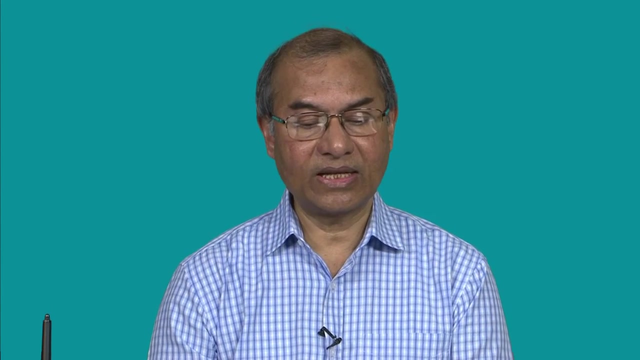 Okay, You understand that this is when we are talking about the aluminum. the aluminum always will have a very quick formation of the aluminum oxide layer and that aluminum oxide layer, like in the case of the cast iron that we have discussed earlier, it will actually serve as a protecting layer on the top of the workpiece and therefore we are saying that the resistance 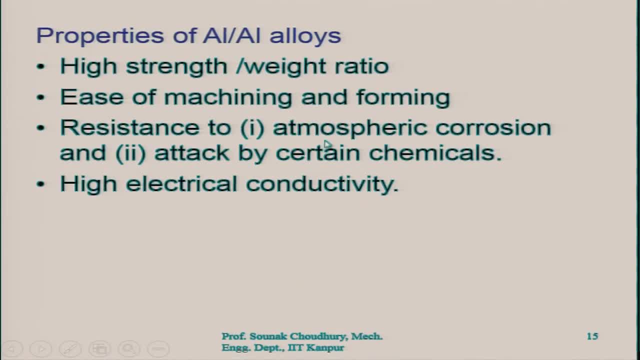 to atmospheric corrosion, particularly atmospheric corrosion resistance high for the aluminium alloys. Pure aluminium, of course, will have a quick formation of the aluminium oxide on top of it, which is harder and attacked by certain chemicals- not all but certain chemicals. Aluminium and aluminium alloys have the high electrical conductivity and for that in the 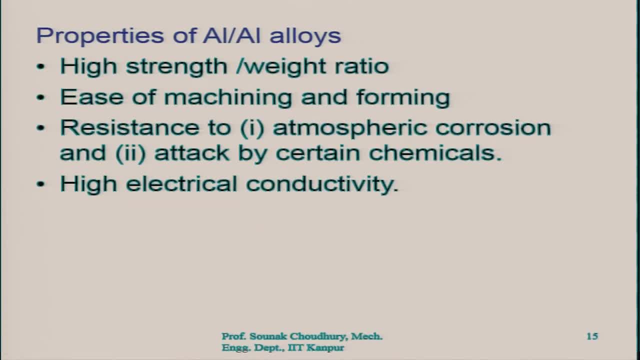 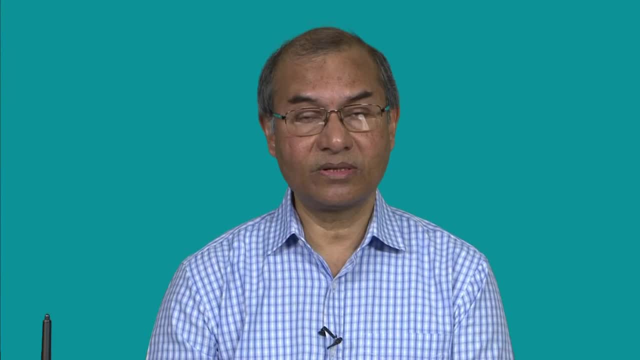 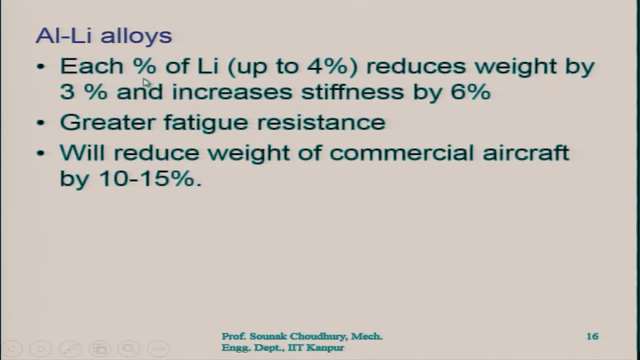 electrical wires also, you can see that there are huge number of aluminium parts and aluminium material, aluminium and aluminium alloys. they are used Now. aluminium lithium alloys, for example. each percentage of lithium, by the way, up to 4% reduces weight by 3% and increases stiffness by 6%. This is the experiment that we have. 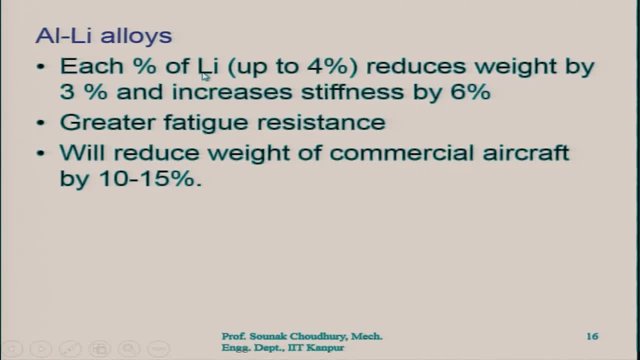 done And you can see the effect. each percent up to 4% reduces weight by 3%. this is drastic reduction in the weight, by the way, and increases the stiffness by 6%. So both these characteristics, like the weight and the increased stiffness, they are desirable in the engineering materials. 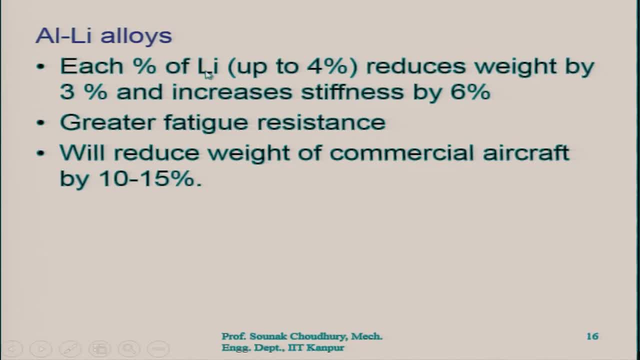 and for the engineering parts. So therefore the role of the aluminium alloys is very important. The role of lithium is great. in case of the aluminium alloy, that has been found out by research: Greater fatigue resistance, so repetitive loads can be withstood by such alloys. aluminium. 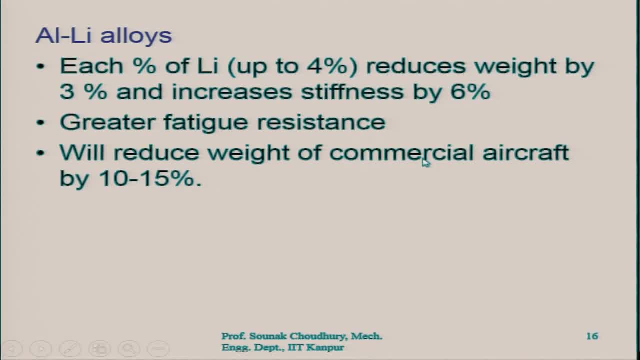 lithium alloys. It will reduce weight of commercial aircraft by 10 to 15%. look at that: 10 to 15% reduction in the commercial aircraft means it is a huge reduction, and the huge reduction not only in the weight but also in the strength of the aircraft. So this is a huge reduction. So this is a huge reduction, and the huge reduction not only in the weight, but also in the strength of the aircraft. So this is a huge reduction and the huge reduction not only in the weight, but also in the strength of the aircraft. So this is a huge reduction, and the huge reduction not only in the weight. 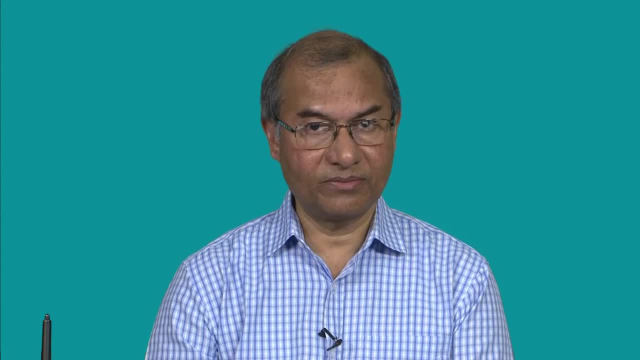 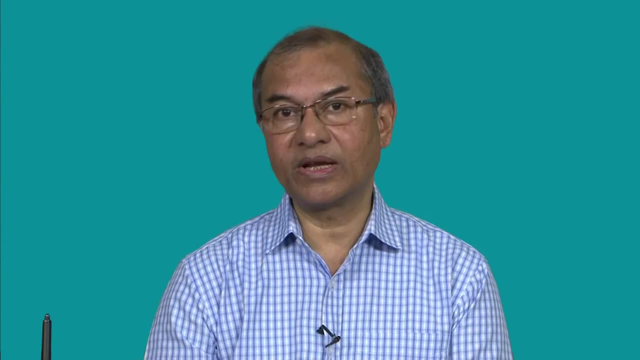 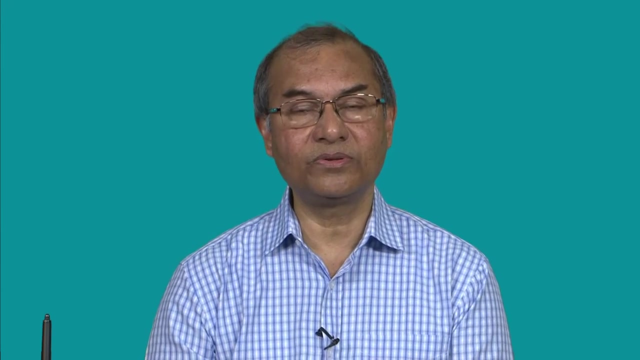 but subsequently in the power consumption. So power consumption means the fuel consumption: Less fuel will be consumed and you understand that in the aircraft the fuel is very, very expensive because very high quality fuel is used. and if the weight is reduced, power is reduced and the fuel consumption is reduced. it is a great achievement for the aircraft. 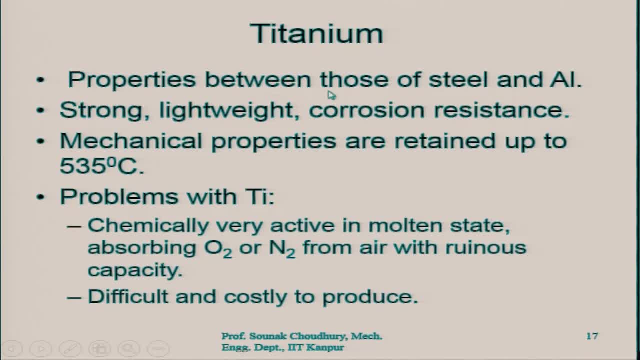 industry Titanium Properties between those of steel and aluminium. So you understand that this is all the properties that the steel have and the aluminium have. The properties of the titanium will be in between. We will tell in details what are those: Strong, light weight, corrosion resistance. These are the three properties which are also 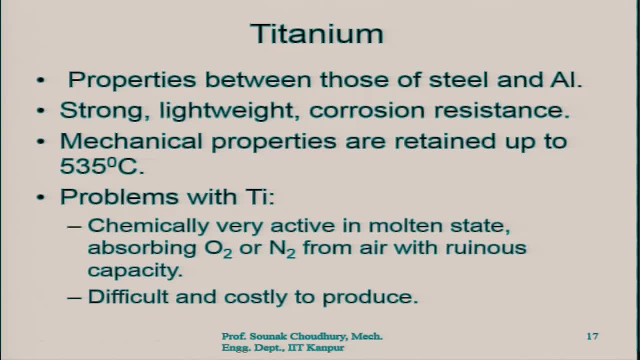 very important for the engineering field of engineering materials. You understand that because they have to be stronger, strong material Weight has to be very high, The weight has to be lighter and it cannot have the corrosion. This should have the corrosion resistance Corrosion. otherwise it will be actually in the long term, the part will be destroyed. 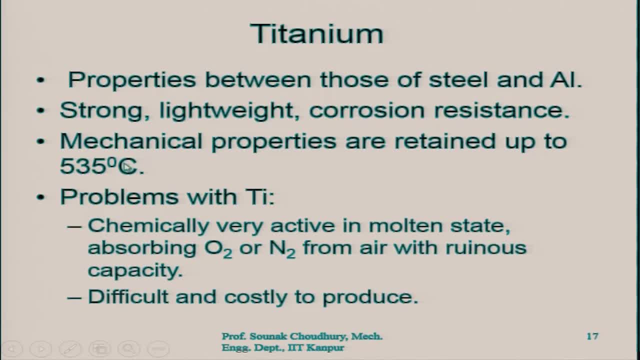 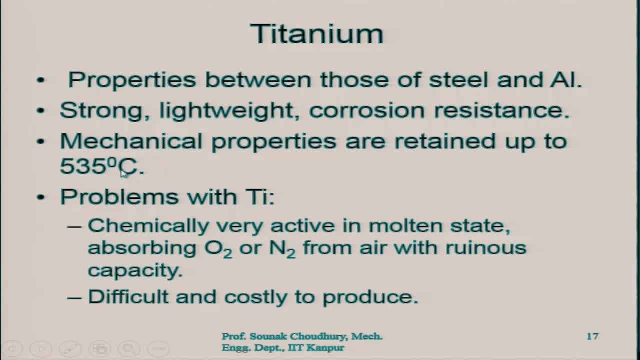 So the hot hardness is reasonably high. I would not say that this is very high, because 535 degree centigrade is not so much high temperature, But still at this temperature the properties, including the hardness, are retained for the titanium parts for which the titanium material is widely used in engineering. 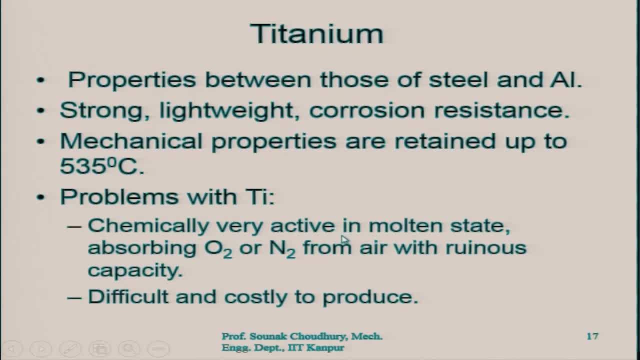 Problems with titanium is that chemically very active in the, particularly in the molten state. Okay, So when it is being produced, when it is being melted, or it is melted for other purposes, for example casting or, you know, for getting the powders and so on, they are chemically. 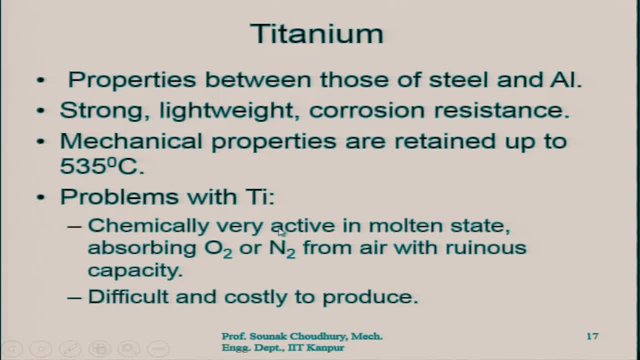 very active. It can react chemically in the atmosphere or the other gases and so on, Absorbing oxygen, particularly, and nitrogen from air with ruinous capacity. So in the molten state particularly, it can absorb oxygen and nitrogen. Okay, So remove oxygen and nitrogen from the air to such extent that it can actually ruin itself. 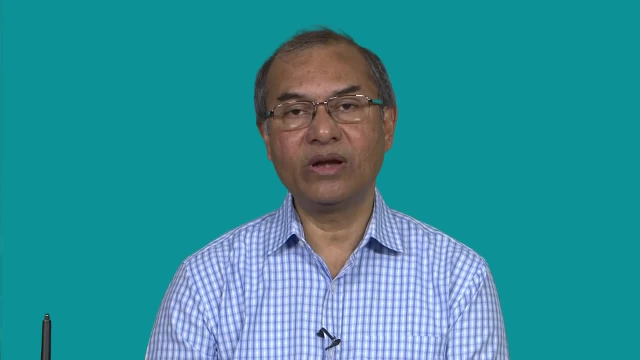 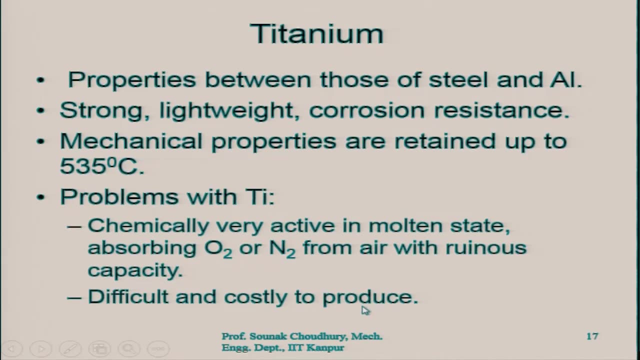 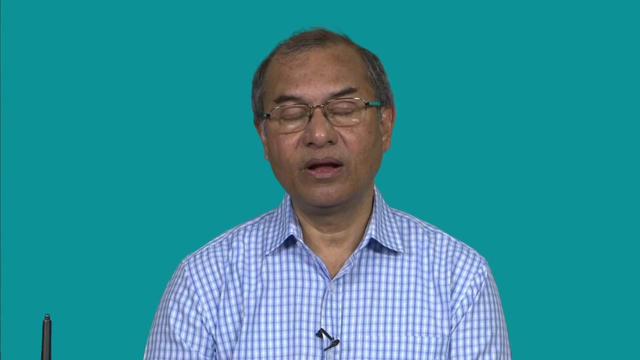 The properties of the titanium can be ruined because of this absorbed oxygen and nitrogen, Difficult and costly to produce. So therefore the titanium material is kind of very rare and it is very expensive. Okay, Modulation in high temperature metals and alloys. 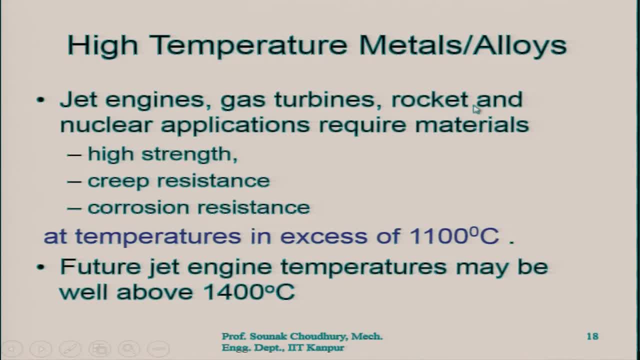 Modulation in high temperature metals and alloys, Jet engines, gas turbines, rocket and nuclear applications. they require the materials with high strength, creep resistance, corrosion resistance. this is understood because you know these are mostly they are working at a very high temperature. that is one thing. 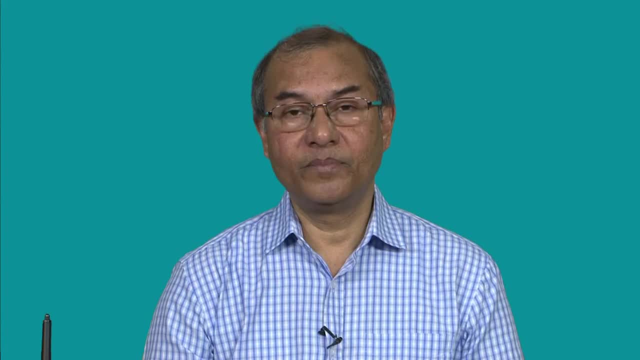 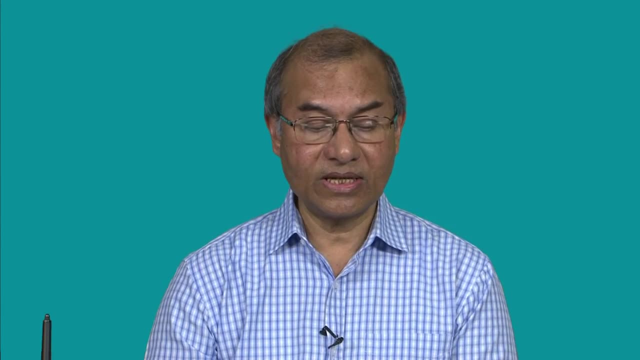 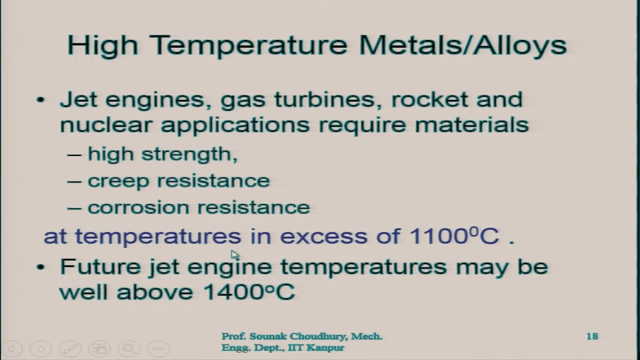 very high speed, So therefore the forces exerted will also be higher. temperature rise will be high. So therefore, for all this it needs the corrosion resistance, creep resistance and the high strength of the material At temperatures in excess of 1100 degree centigrade, so the temperature may go, of course, more than. 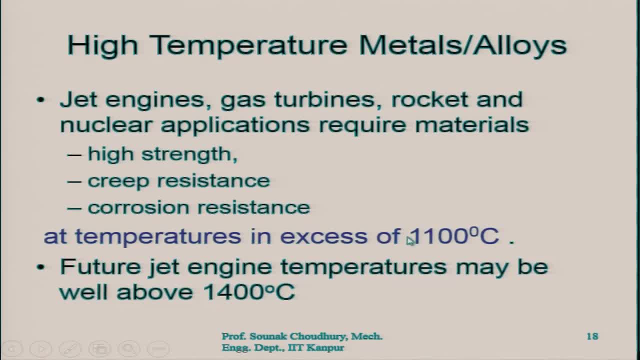 1100 degree centigrade. So at this temperature all these properties should be retained. That is, high strength, creep resistance and corrosion resistance. See the important point for these parts or this material for the jet engine, gas turbine and so on. it is not only the overall properties, but we always ask that these properties should. 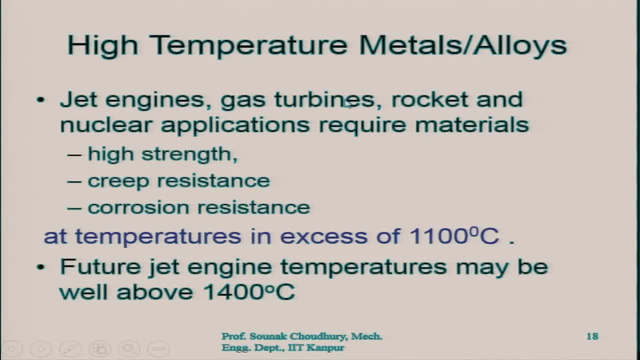 be retained at higher temperature because mostly in the jet engines, gas turbines, rockets, nuclear applications the temperature goes beyond this 1100 degree centigrade. alright, So at that high temperature When these properties are retained, that is valued and that is desired, okay. 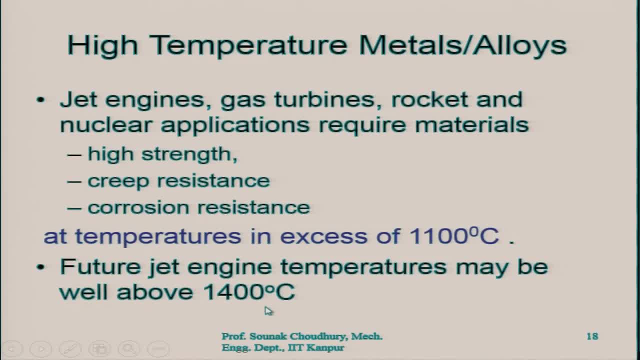 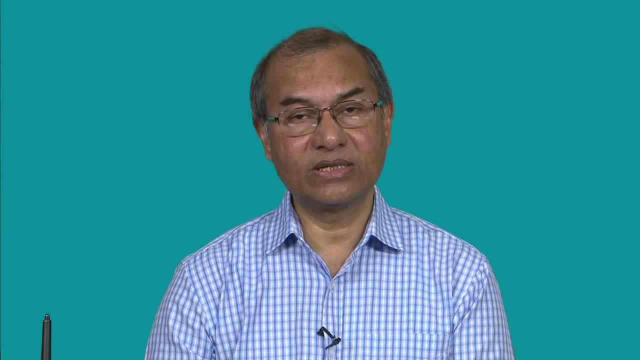 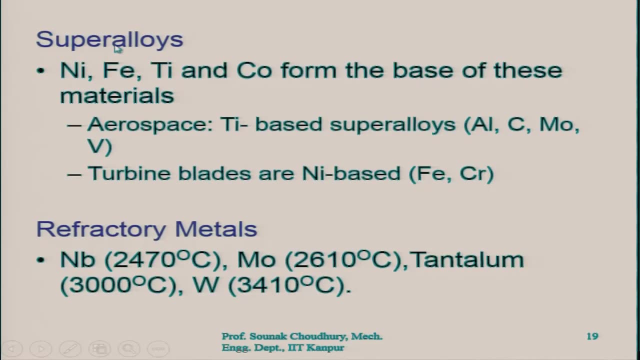 Future jet engine temperatures may well be above 1400 degree centigrade, because the speed is increased and therefore the temperature is increased and the forces exerted on them also are increasing. okay, Therefore, materials like super alloys are invented. Nickel Ferrous. 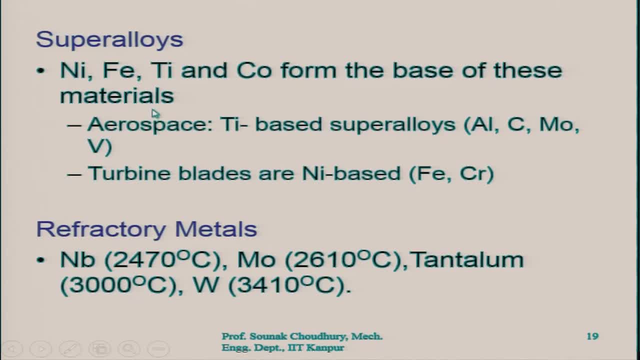 Titanium and cobalt form the base of these materials. These are the super alloys formed by nickel, ferrous titanium and cobalt In aerospace, particularly the titanium based super alloys, for example, aluminium made of aluminium, carbon molybdenum, vanadium, along with the titanium okay. 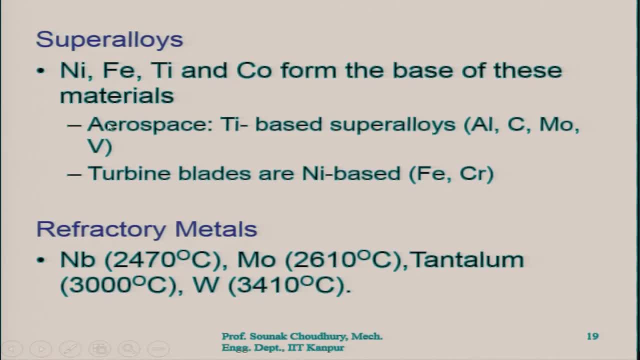 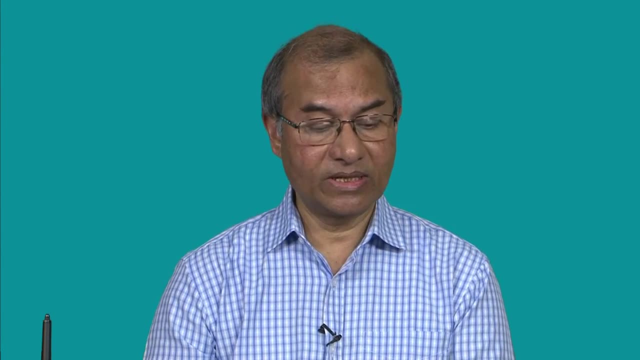 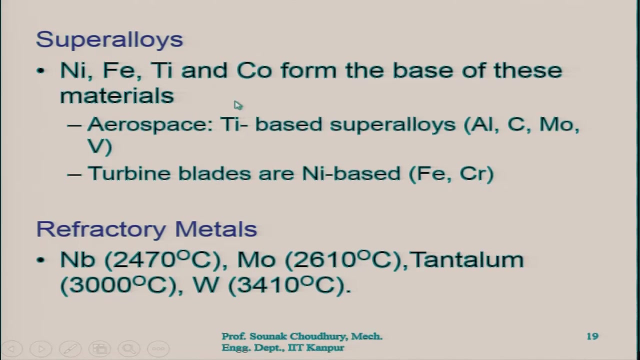 Titanium will be the base That is very widely used in the aerospace, Particularly because they become very light- okay- and strength wise. also, it is sufficient for the parts made in the aerospace industry. Turbine blades are mostly nickel based, along with the ferrous and the chromium. 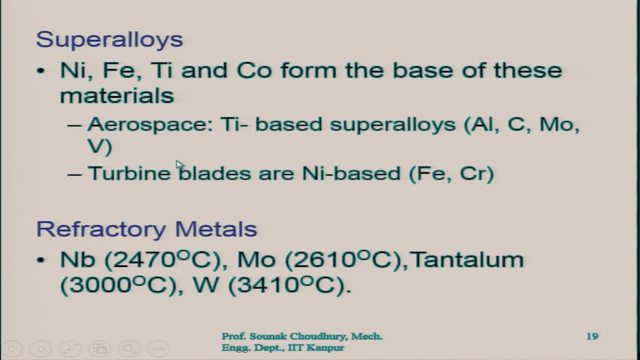 So these are the super alloys which will have superior properties that are required and used in the aerospace or the aerospace industry. Okay, In aerospace industries, particularly because turbines mostly are used in the aircrafts, all the engines, you understand that. and there the super alloys are used for making the blades. 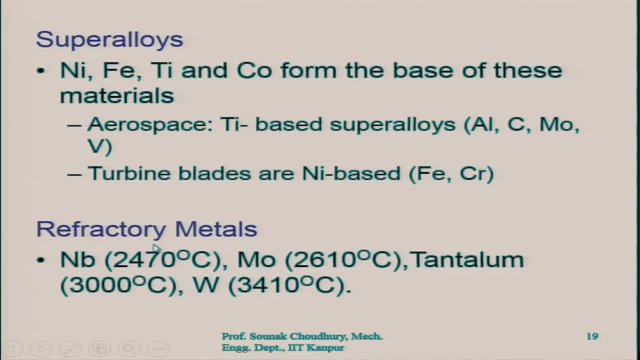 making the housing and so on. Refractory metals: niobium- I suppose this is 2470 degree centigrade, it can actually withstand. Molybdenum can withstand 2610 degree centigrade. Okay, So these are the super alloys. 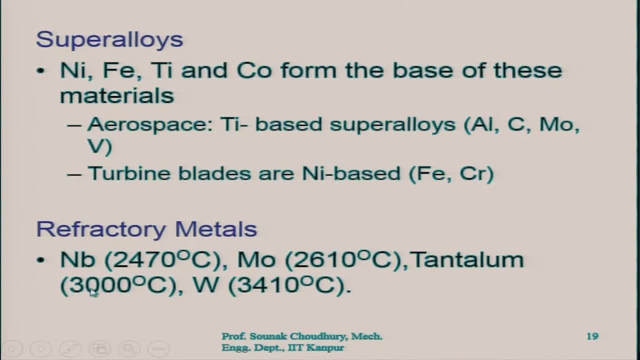 Tantalum can withstand even more, up to 3000 degree centigrade. or tungsten can withstand 3410 degree centigrade. So the refractory metals, you know that those metals are used for making the layers in the furnace. okay, in the where you have you melt, we get the molten material. 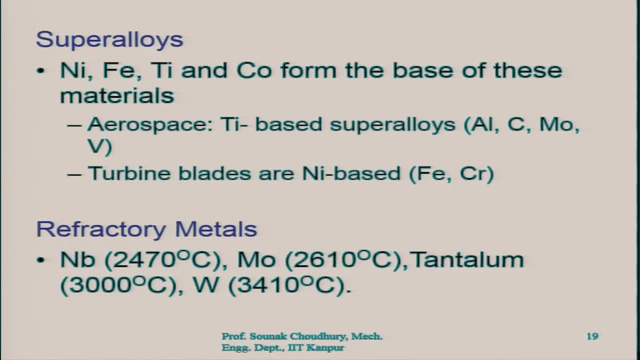 We prepare the steel, prepare the steel. I mean alloys. alloys are used for making the alloys. Okay, I mean alloys alloying materials. okay, alloy steels and so on. So there the temperature becomes very high and we cannot have any loss in the temperature. 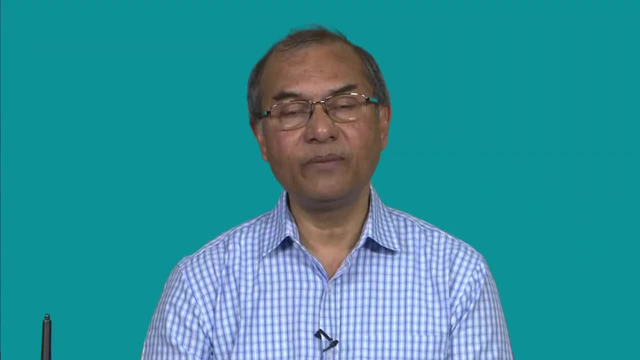 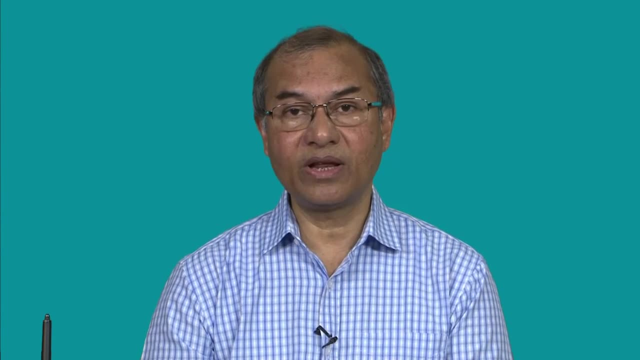 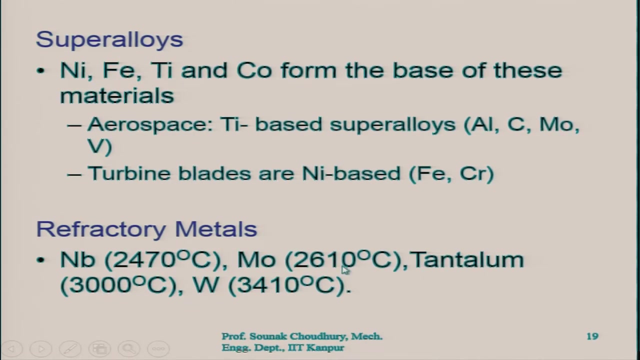 So, therefore, inside those furnaces there is a layer which is made by the refractory metals, And the refractory metals, therefore, should withstand very high temperature, and you can see that these materials actually can withstand really high temperature, which is beyond the melting temperature of many metals. actually, 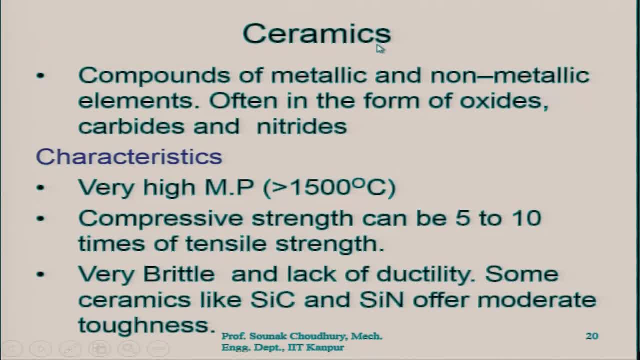 Ceramics, compounds of metallic and non-metallic elements. these are the ceramics, often in the form of oxides, carbides and nitrides. okay, So there are different kind of oxides, different kind of carbides- we will see this- and the nitrides, which are actually the ceramics, which are called the ceramics. 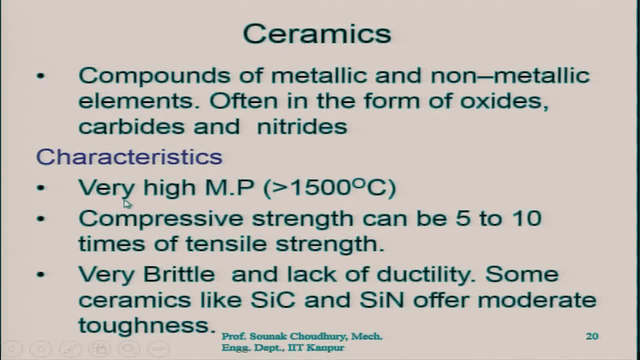 Now, the characteristics of the ceramic are that they have very high Melting point. melting point is more than 1500 degree centigrade. So therefore, at very high temperature, like up to this temperature, it cannot melt. okay. Compressive strength can be 5 to 10 times of the tensile strength. okay. 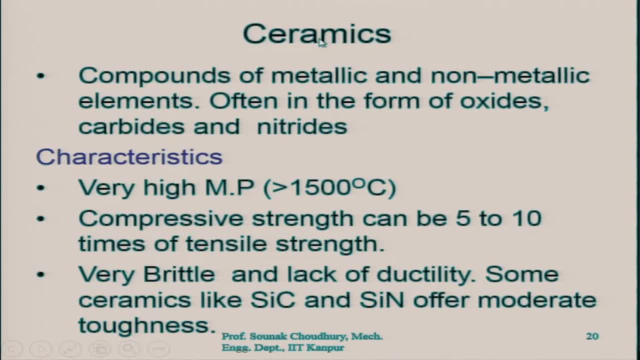 Here, as you understand that these materials are the brittle materials- ceramics- okay. So therefore their tensile strength is not high, But the compressive strength is very high. Okay, This is even 10, up to 10 times more than the tensile strength because of that property. 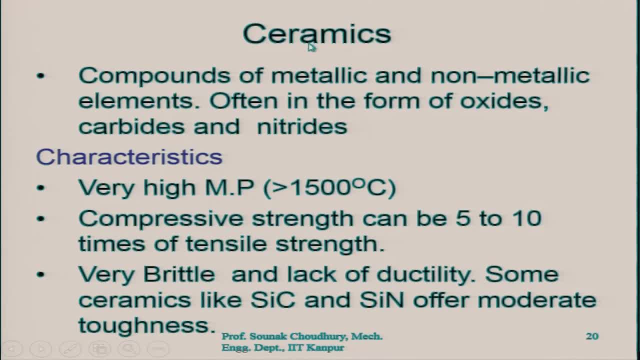 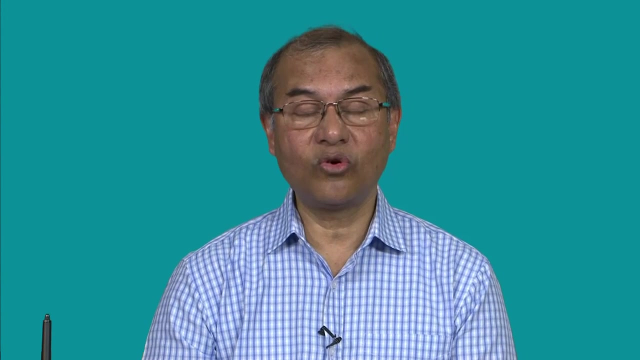 actually, because of the high compressive strength, these ceramics are very often used widely. Very brittle and lack of ductility. okay, Some ceramics like silicon carbide, silicon nitride. they offer moderate toughness. They can reasonably well withstand the shocks. okay. Now ceramics are overall not very good shock absorbers. 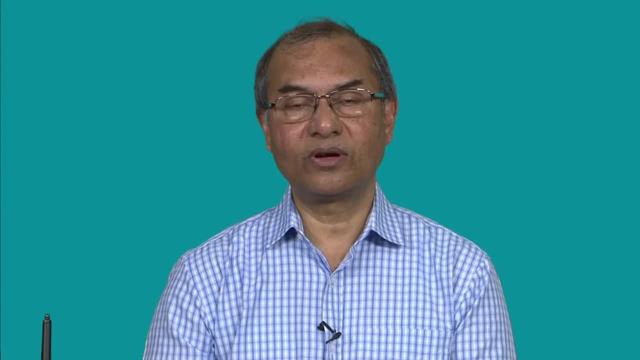 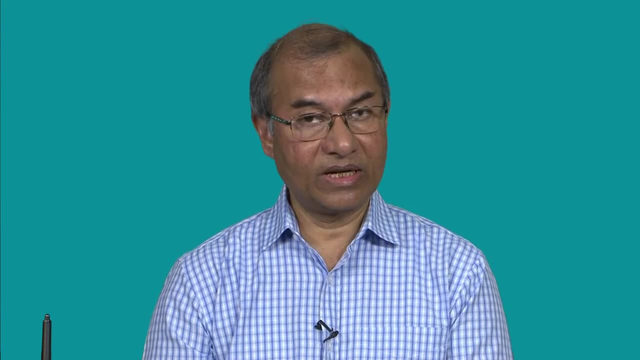 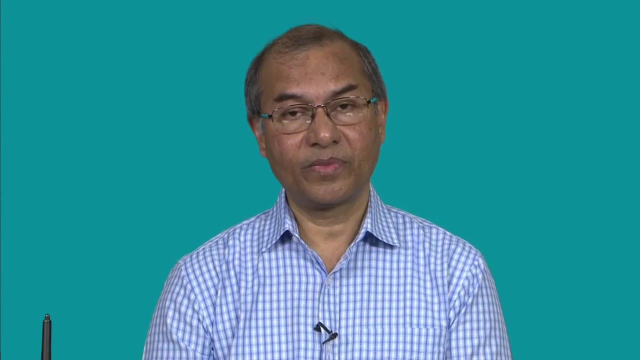 If you have a. let us say, for example, in case of tools, in case of tools in machining, the tools are made of ceramics, But those tools cannot withstand the vibration in the machine tool. okay, If the tool vibrates, then the ceramic tools actually can break. 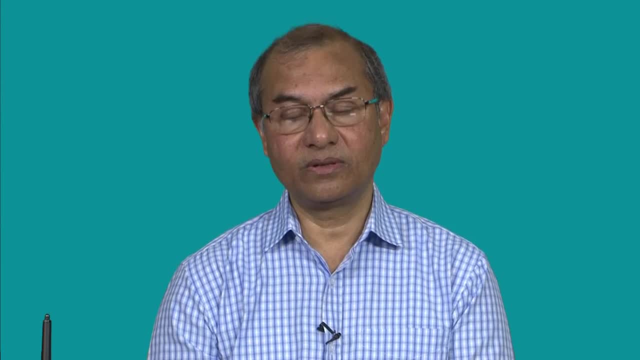 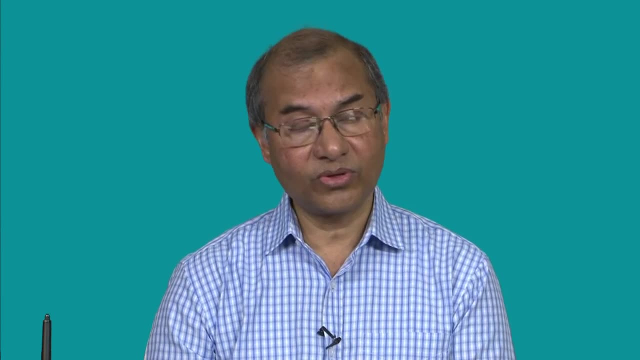 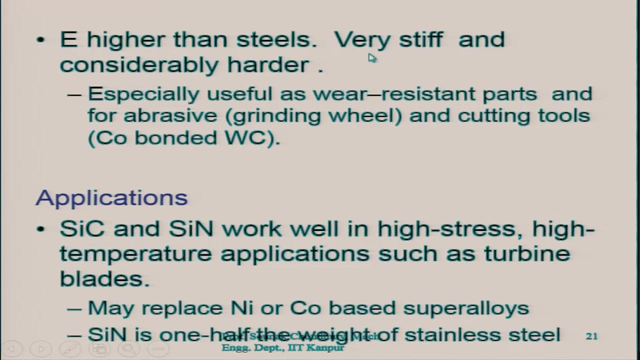 All right. So therefore, In case of turning tools, the ceramic tools are made fatter so that they can actually withstand the high- I mean fluctuation of force- particularly okay. That is not very good for ceramics. Young's modulus: higher than the steel, very stiff and considerably harder okay. 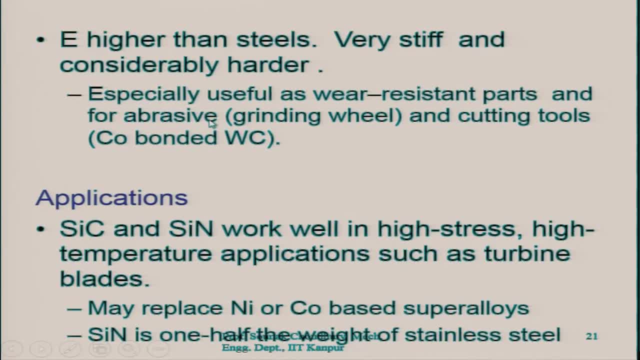 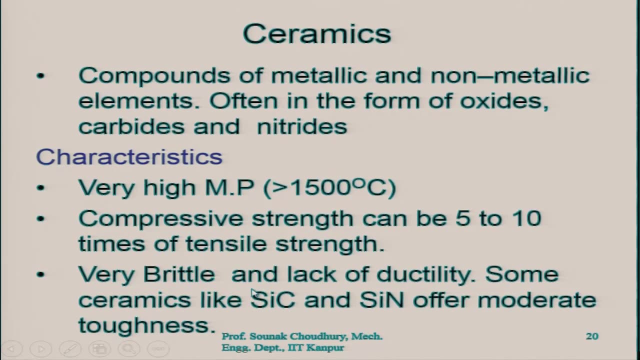 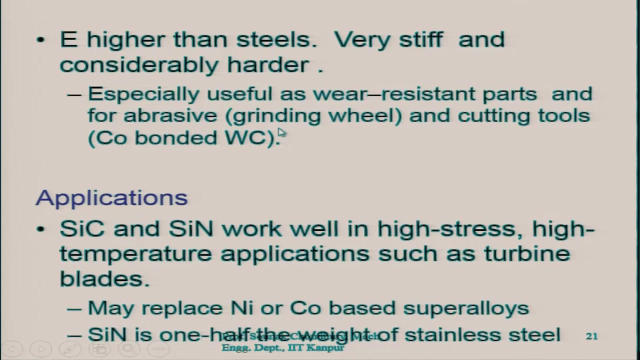 Especially useful as wear resistant parts and for abrasives, like very often ceramic particles are used In terms of silicon carbide, for example. okay, So we said that silicon carbide, silicon nitride, they have the moderate toughness. okay, So those silicon carbide particles are also used as the grinding wheel grids. okay, 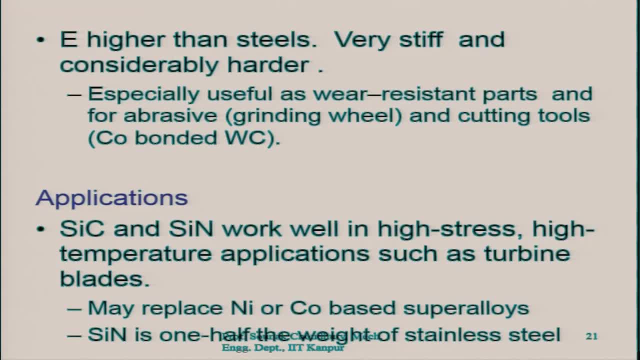 So that we will discuss, when we will discuss the machining part in the conventional machining, that grinding wheels are very wide, very widely used. the abrasives, okay, Okay, This kind of abrasives like ceramics, So particularly the silicon carbide Cutting tools. very often cutting tools are of the tungsten carbide. 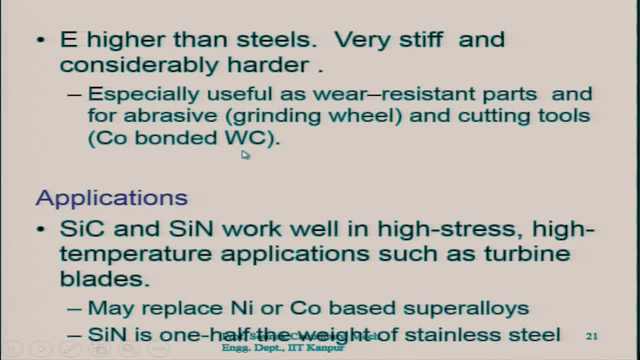 They are very strong and they cannot withstand. of course they are brittle, as I said, but they can withstand very high temperature and they have the quite a good wear resistance. all right, So this is. the tools do not wear out very easily when they are made of the tungsten. 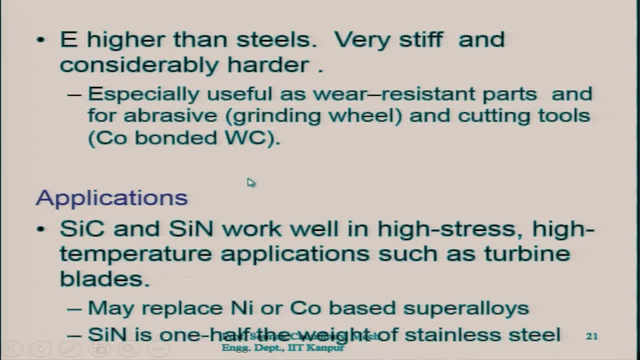 carbide. Tungsten carbide is a co-bonded okay with the tungsten carbide Applications. silicon carbide and silicon nitride work well in high stress when the stress is high, High temperature applications such as turbine blades. So blades are made of the along with the silicon nitride and the silicon carbide as well. 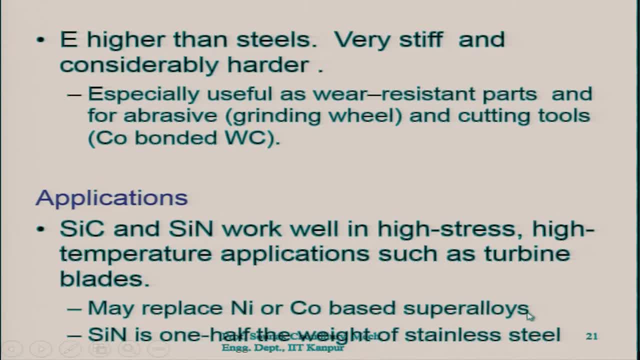 May replace nickel or cobalt based super alloy Be made, Because the properties of the ceramics will be closer to that those super alloys- nickel or cobalt based super alloys. Silicon nitride, for example, is one half the weight of the stainless steel. okay. 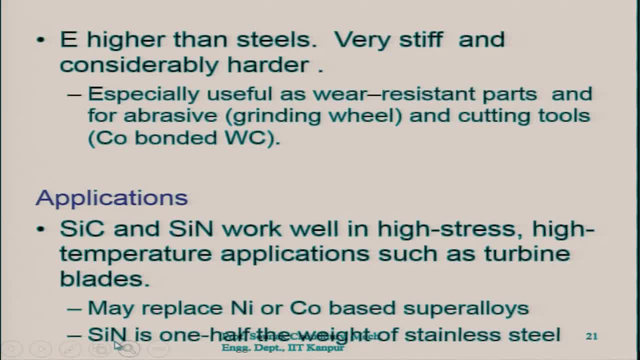 So you can understand that these are much lighter materials also. So if you are using the stainless steel, the structure will be much heavier than the use of the silicon nitride. Okay, But in case of silicon nitride, of course it is more expensive than the stainless steel. 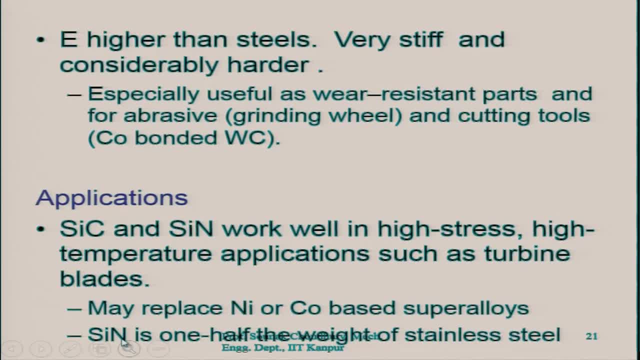 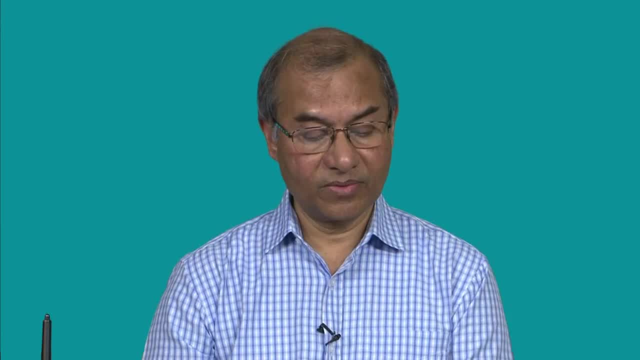 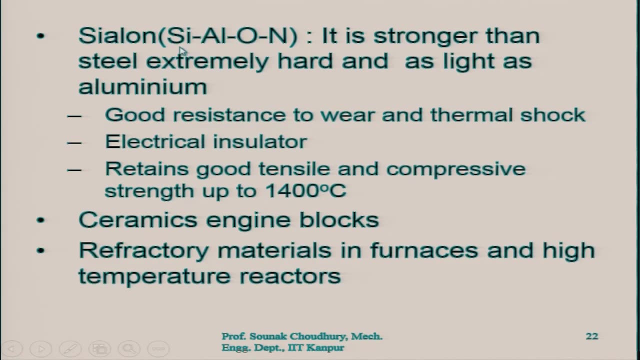 But where you have the weight as a factor. in that case you have to. you cannot compromise with the property and you have to go for the high cost of the silicon nitride. Okay, Cialon, for example. this is a relatively new material and I will just tell you the definition. 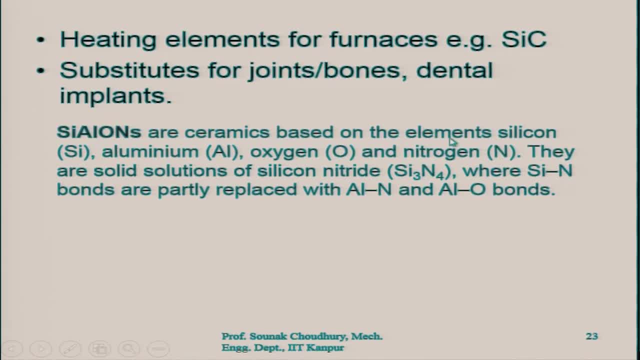 of that. The cialons are ceramics based on silicon nitride. Okay, Cialon, for example. this is a relatively new material and I will just tell you the definition of that. The cialons are ceramics based on silicon nitride. 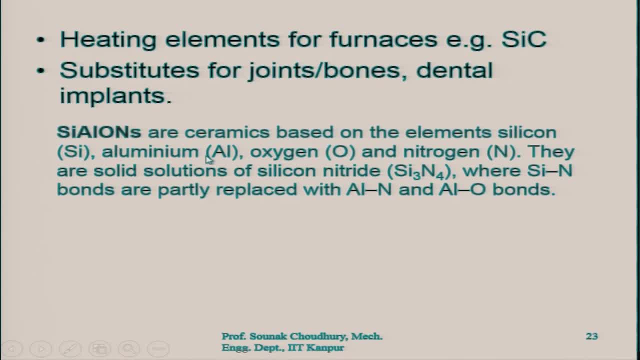 Okay So the cialon is based on the elements silicon, aluminum, oxygen and nitrogen. that is why the name came silicon, aluminum, oxygen and nitrogen. Okay So, cialon, they are solid solutions of silicon nitride, Si 3N4, where silicon nitrogen bonds. 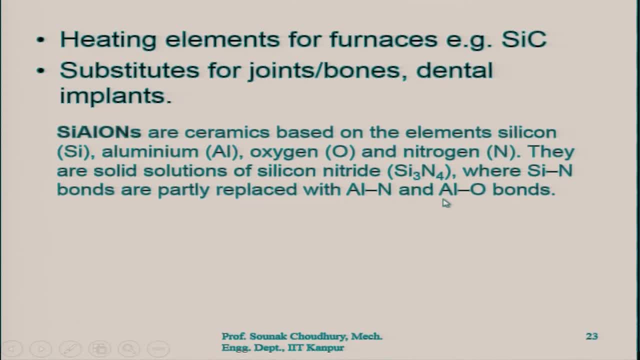 are partly replaced with the aluminum nitrogen and aluminum oxygen bonds. this is how the cialon has been invented, been invented that silicon nitride, silicon nitride, these bonds. they are partially, partly replaced by the aluminum nitride, aluminum nitrogen and the aluminum oxygen bonds. 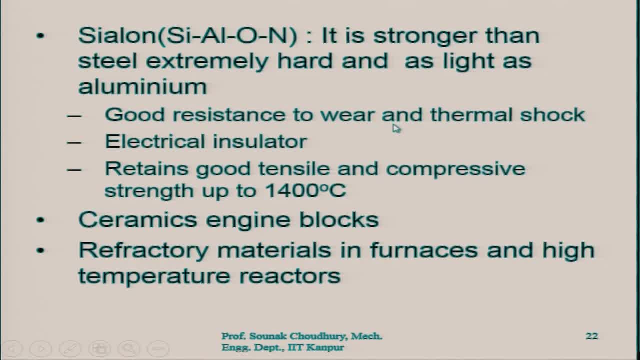 Now they have good resistance to wear and thermal shock. It is stronger than steel, by the way, extremely hard and light as aluminum. So you could see the extremely good properties like stronger than steel, okay, extremely hard, light as aluminum. So the meaning that it is using the all the good properties of the steel aluminum materials. 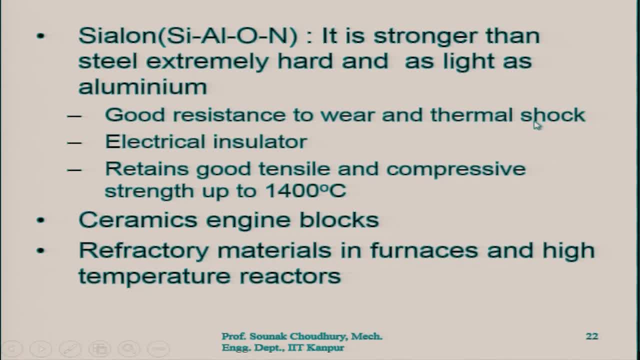 So good resistance to wear and thermal shock, as I said, It has the electrical it good electrical bad conductor, so it can be used as an insulator. okay, retains good tensile and compressive strength, particularly up to temperature of 1400 degree centigrade. 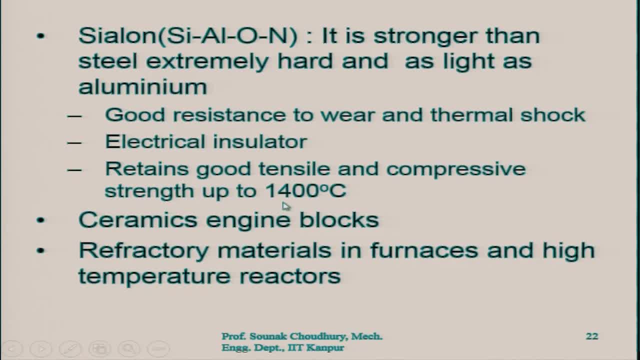 It is a very high temperature, you can see that, and it at that temperature it may have the tensile and the compressive strength to retain. okay, Ceramics engine blocks are also coming up. okay, So that is, ceramic material is used for making the engine blocks as well. 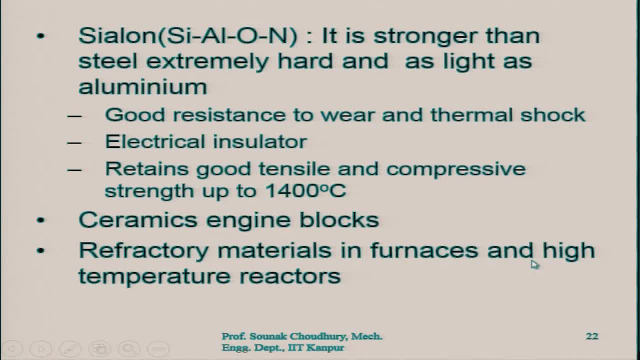 Refractory materials in furnaces and high temperature reactors. they are used because they can actually withstand very high temperature. They can retain good tensile and compressive strength. So therefore in the engine blocks, in the refractory materials in furnaces, okay, So they are used as this kind of material. 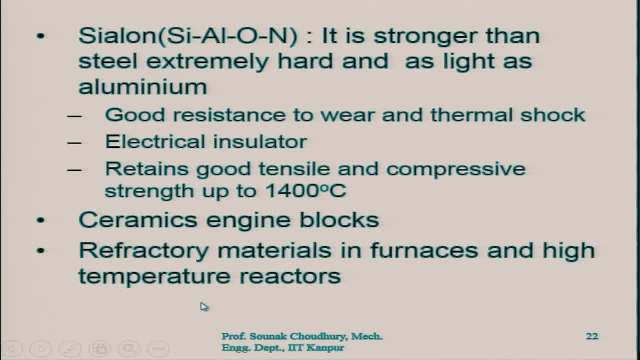 So in engine blocks, of course it is a layer. Okay, It is not full. engine block material could not be from the ceramics. okay, So it is a layer. and inside the engine block, which is of the Cialon material, It is also ceramic material. 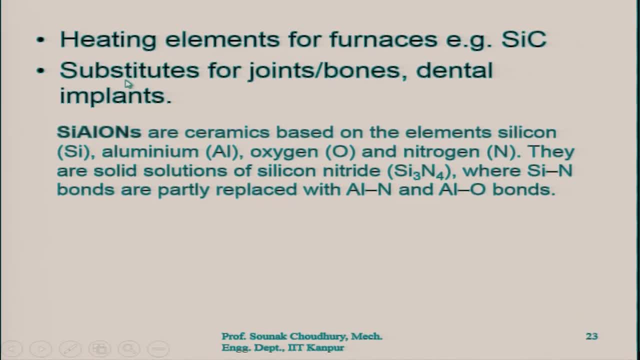 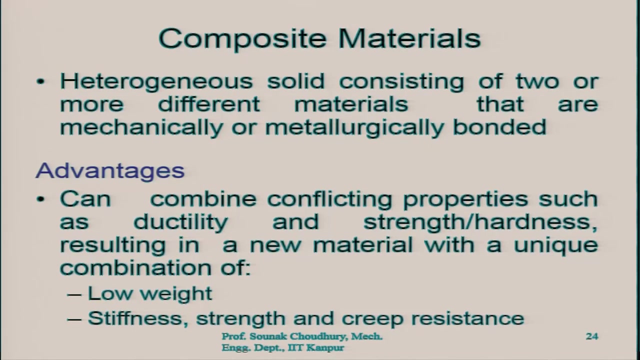 Heating elements for furnaces, for example, silicon carbide. okay, Substitutes for joints, bones, dental implants. this material is now being more and more popularly used in the dental implants and the substitute for the joints. okay, Now composite materials. as I was telling you that this is, these are the materials which 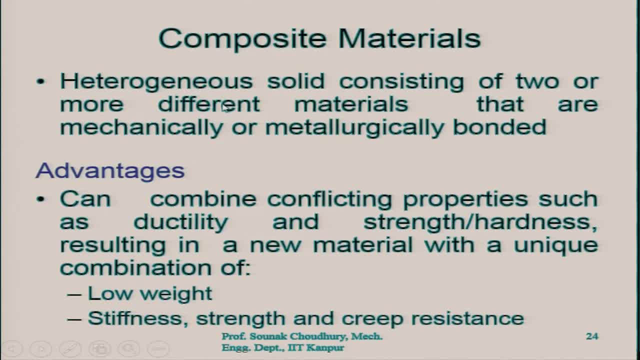 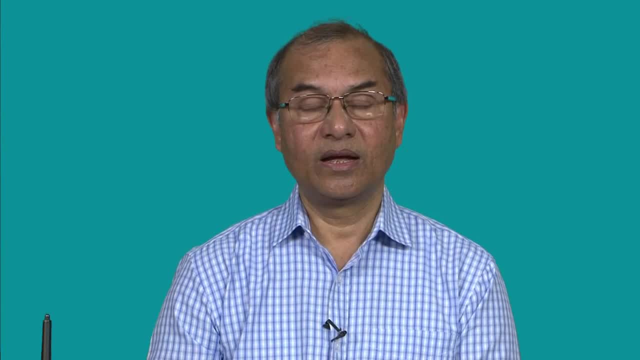 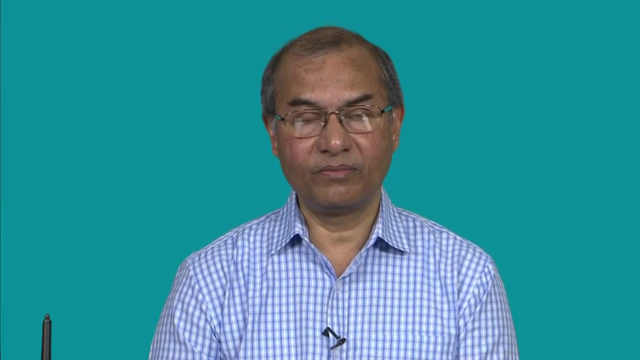 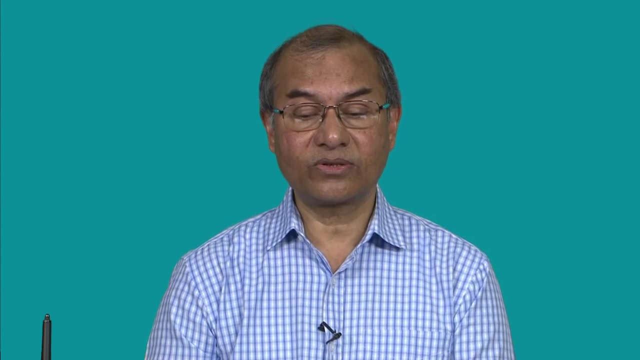 have lately started being used very extensively because of their unique properties, particularly the light and strong okay, And they are relatively less expensive. They can be, they can be made, produced easily, and so on. relatively easily. Heterogeneous solid consisting of two or more different materials that are mechanically 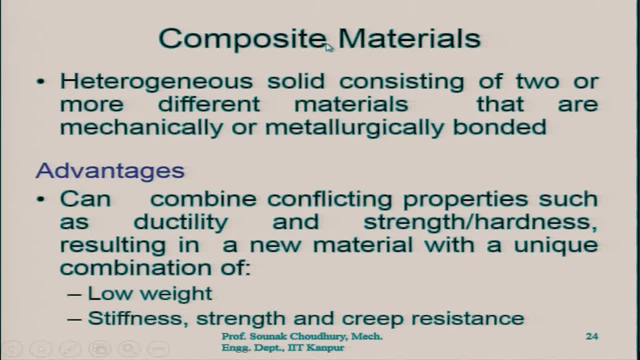 or metallurgically bonded. These are the composite materials. Once again, these are the heterogeneous solid okay, and they consist of the two or more different materials That are mechanically or metallurgically bonded. we will see how they. what does it mean that mechanically and what does it mean metallurgical bond? 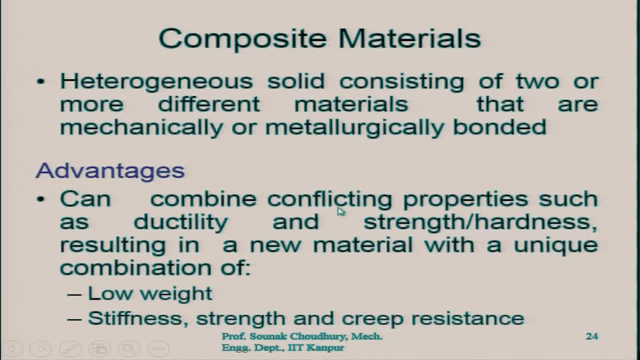 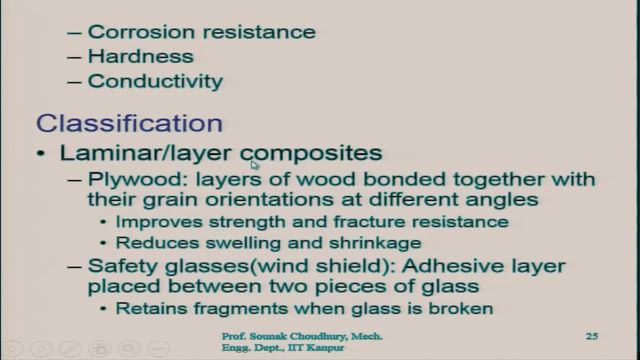 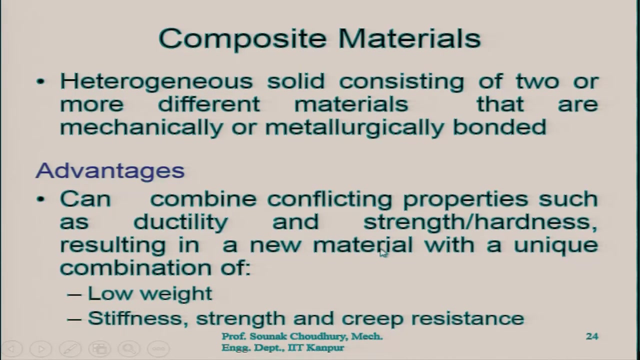 Advantages of the composite materials are that they can combine conflicting properties such as ductility, strength and hardness, resulting in a new material with a unique combination of low weight, stiffness, strength and creep resistance, corrosion resistance, hardness and conductivity. You can see that in case of the material, if you have a hard material, normally they are. 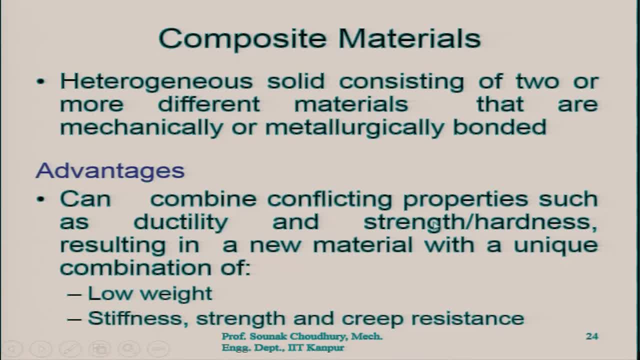 brittle, okay. So if you have the strength- high strength- though- they may not have the ductility. If you have high hardness, they may not, they will not have the ductility, and so on. So in case of composite material, this is the advantage: that it can combine these conflicting 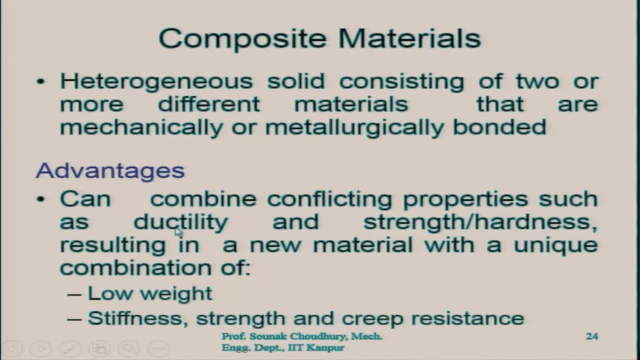 properties: okay, It can have the ductility as well as the hardness, for example. These are the unique properties which are desired in the engineering materials. okay, to make the engineering parts, which needs very high hardness, and they should be also ductile to a certain extent. 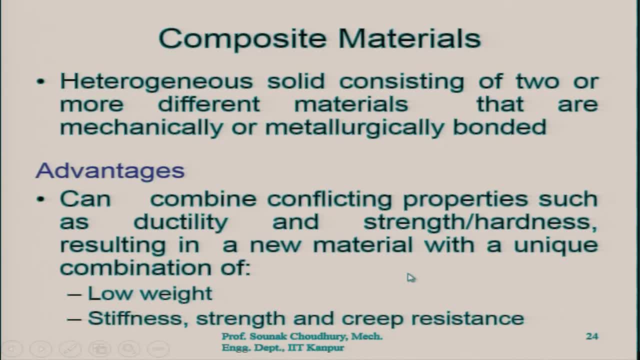 I will give you examples in the course of our discussion, that we need to have the parts, we need to have the tools, even which will have the hardness as well as the bit of hardness. So these are the unique properties. Okay, Now, as I said that they are, these composite materials, therefore, are of low weight stiffness. 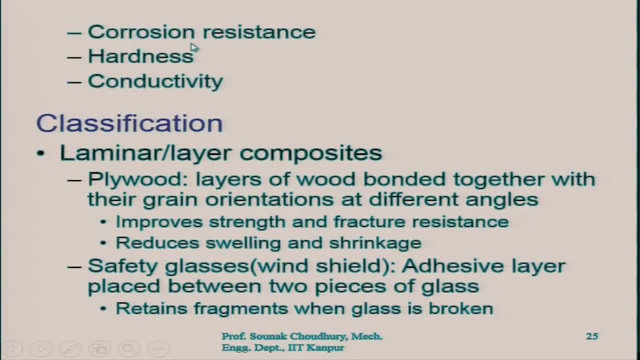 strength and creep resistance. high corrosion resistance is high, high hardness and high conductivity. okay, Now the classification in the you know composite materials are that laminar? it may be laminar or layer composites as it is said, For example Plywood. 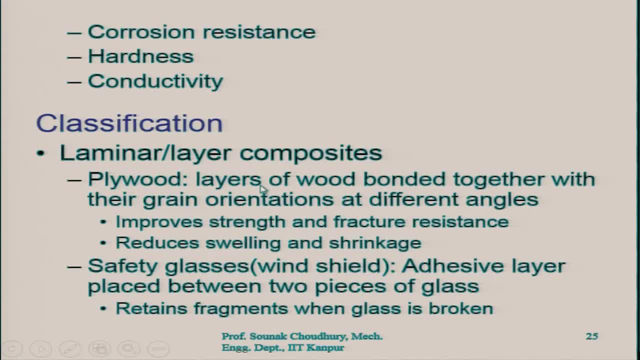 Plywood, Plywood, Plywood. they have the layers of wood bonded together with their grain orientations at different angles. okay, so this is called the Plywood. This is also kind of a composite material. alright, improves strength that way, because it has the grain orientation. depending on the grain orientation, they are actually those. 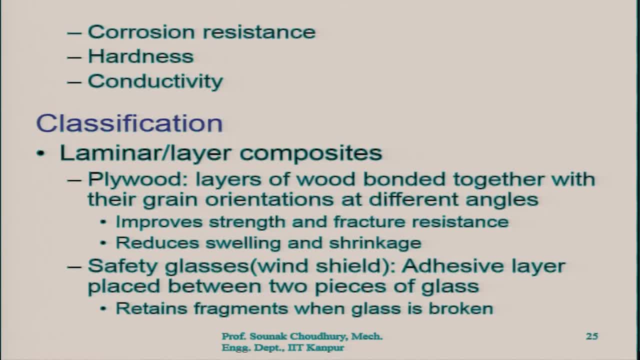 grain orientations are at different angles. so therefore, depending on that, you can actually gain the particular strength. you can obtain the particular strength and the fracture resistance. It cannot actually fracture very easily, all right, Reduces swelling and the shrinkage. so this is very important, particularly for the household. 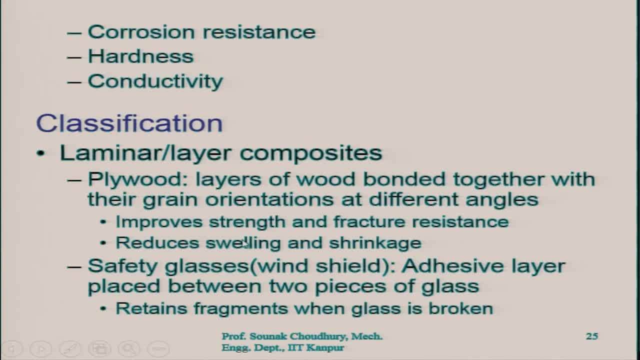 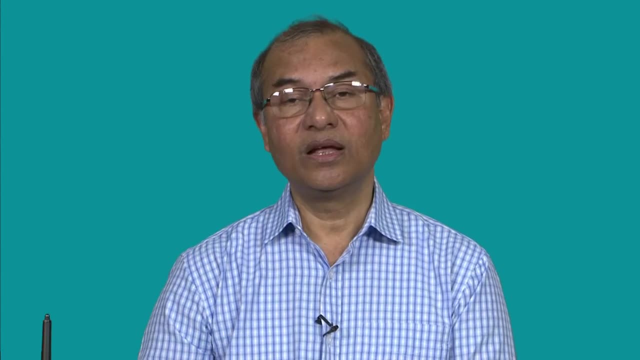 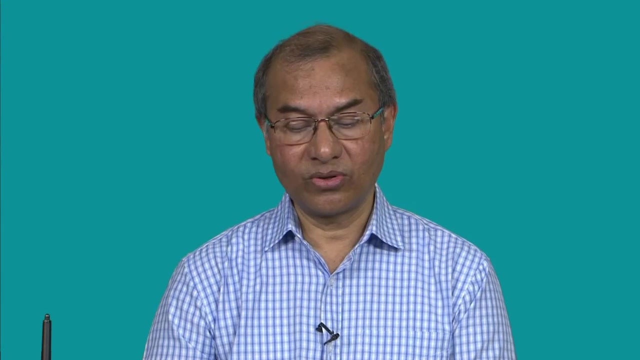 doors and windows, as you understand that under the rain they should not swell or they should not shrink. at a higher temperature or at when the humidity is less, for example the dry condition, they should not shrink. In that case you understand that the doors and windows and all household furnitures, 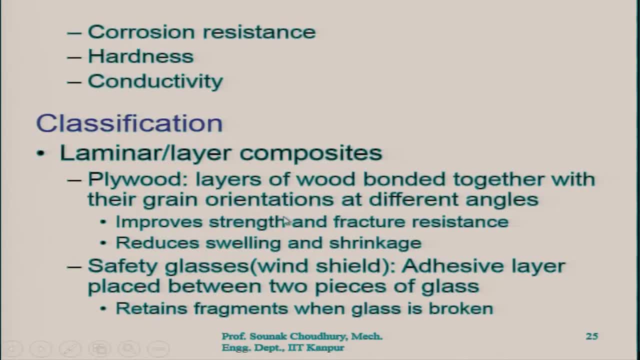 and all they will suffer. So this is the plywood, which is also a kind of a composite material: Safety glasses, windshields, for example- okay, Adhesive layer placed between two pieces of glass. So this is how the safety glasses or the windshields are made. all right, 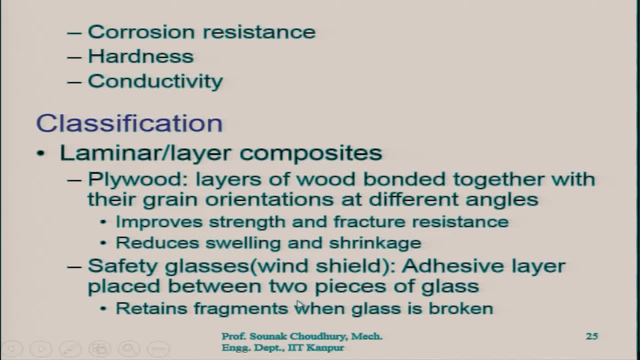 Because they have the adhesive layer so they cannot actually break in pieces, but they retains the fragments when the glass is broken. this is important. You might have seen that if a tone falls at the windshield of an automobile, it does not actually come out okay. 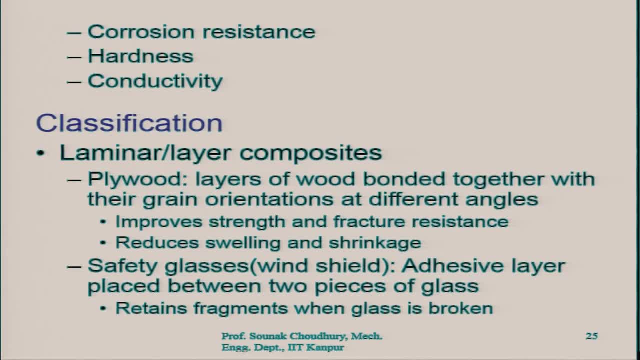 It does not break. It does not break into pieces, It actually breaks and stays there. the pieces can stay there all right. So this is done by the adhesive layer placed between the two pieces of glass. this is how the safety glasses are made. 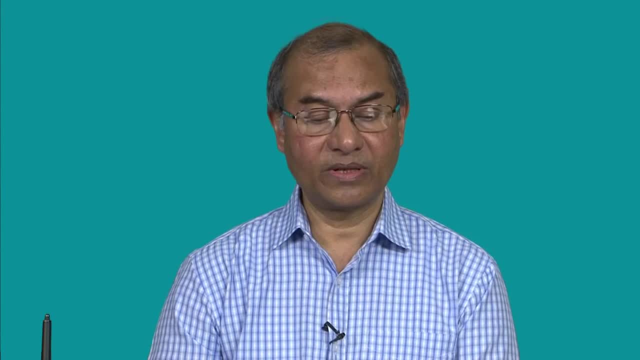 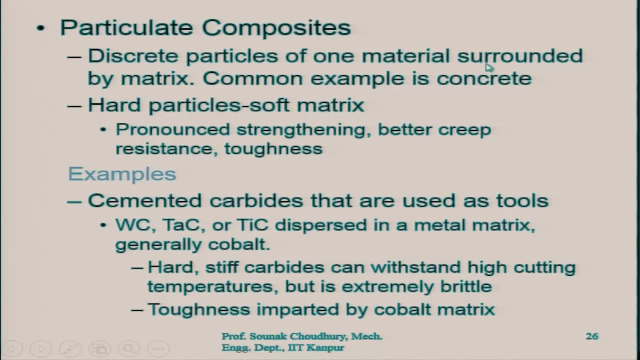 So this is also a kind of a composite material. okay, as per the definition, Particulate composites are there. Particulate composites are the discrete particles of one material surrounded by matrix. okay, Common example is a concrete. It is a discrete particle of one material. which material? it is a cement, for example. 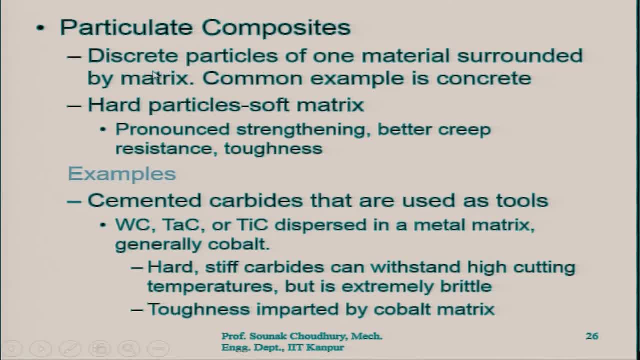 surrounded by matrix. okay, So this can be the cement and the granules. okay, that makes it. and the sand, for example, So that will be the concrete Hard particles, soft hard particles, soft matrix- okay, So pronouns strengthening better creep resistance. 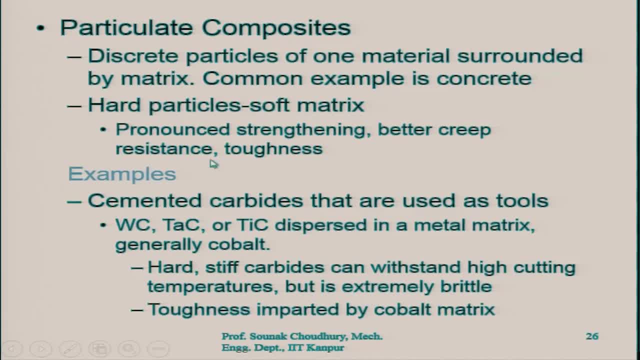 Okay, Hard resistance, toughness, all right. Examples: they are the cemented carbides that are used as tool, For example, tungsten carbide, tantalum carbide, titanium carbide- okay, dispersed in metal matrix. So these are the cemented carbides. as you may remember that, these are the materials. 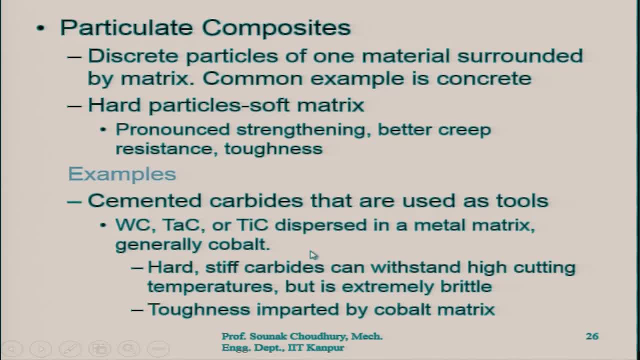 also they are used for making the tools- okay, cutting tools Generally. Generally, that metal matrix used there is the cobalt. okay, So the cobalt metal matrix and the powders will be tungsten carbide, tantalum carbide and the titanium carbide. all right, 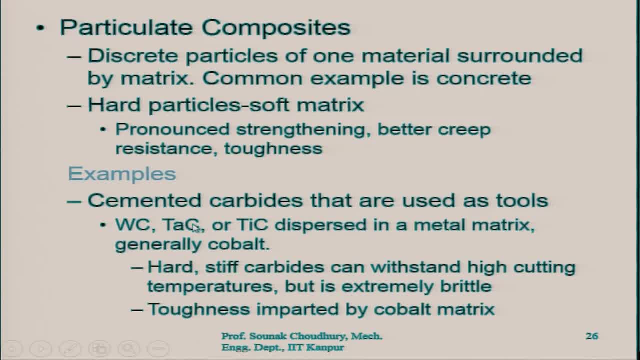 As a result, you will get the unique properties that we have discussed: High strong material. it can withstand the shock loads- okay, it can withstand the fatigue, and so on. Hard, stiff carbides can withstand high cutting temperature- Okay, High cutting temperatures. that is very important. 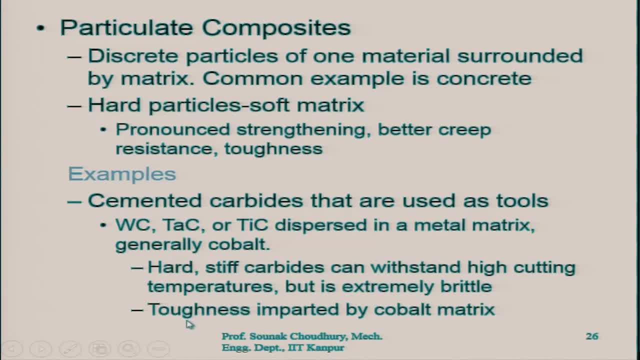 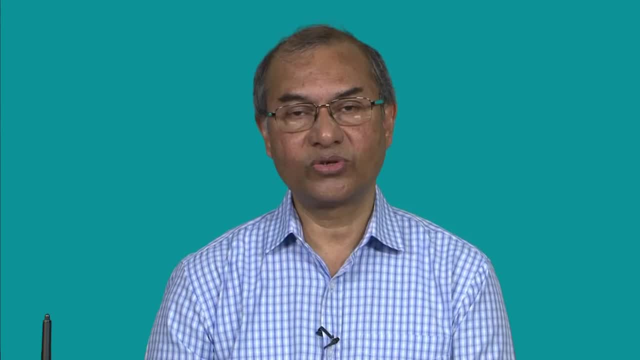 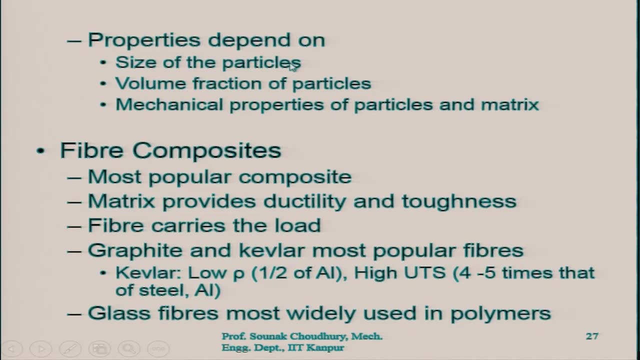 But extremely brittle. okay, Toughness imparted by the cobalt matrix. So cobalt matrix improves that shock absorption property to an extent. all right, Properties also depend on the size of the particles, of course. Volume, fraction of particles, that means how much which particles are in which volume. 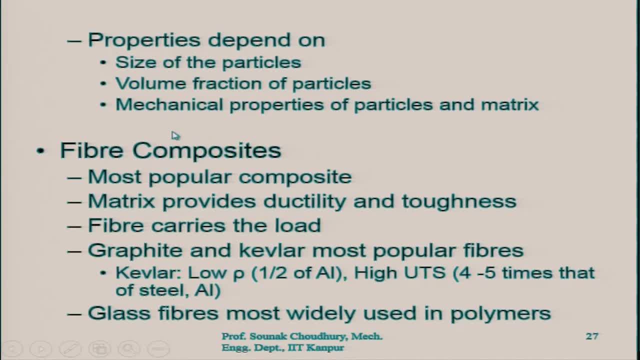 in the. what is the fraction of this volume? okay, Fraction of this volume, Fraction of those particles in that volume, and the mechanical properties of the particles and the matrix, both okay. So in the composite material the properties of these particles or the matrix may not be. 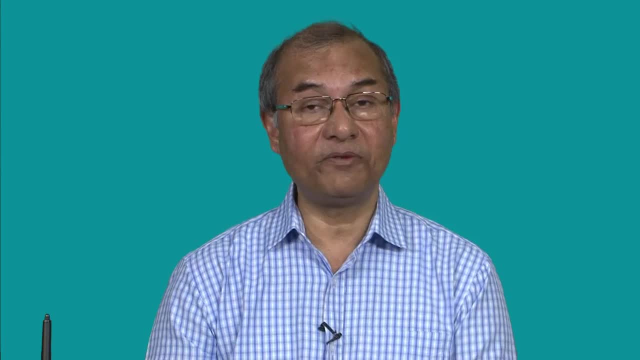 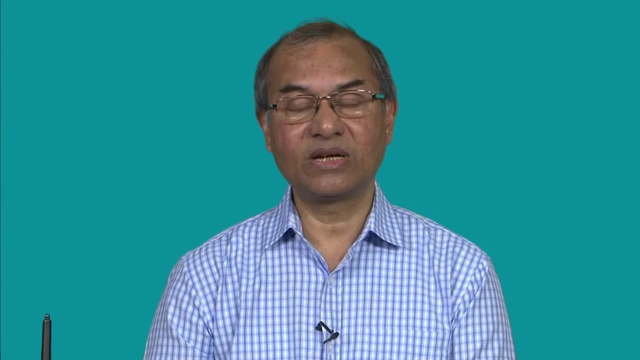 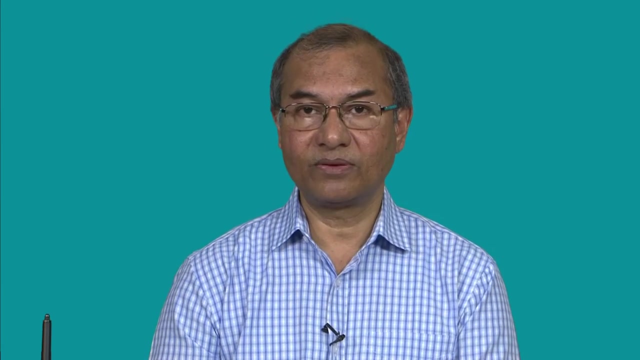 retained. okay, The properties may be different and the properties normally are better than the properties of the particles and the matrix taken individually. Okay, So it is like case of the mixture, when you are making two liquids also. So it happens, you know that. 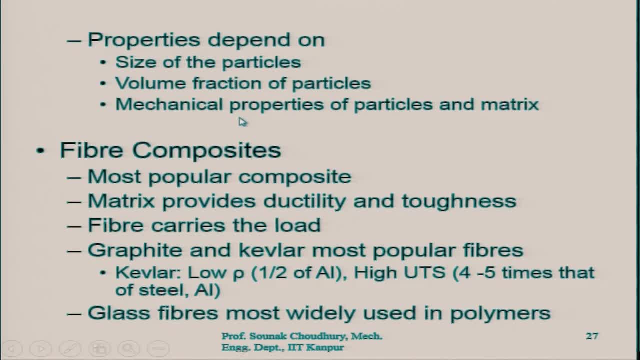 And therefore the composite material, the properties that you are getting will be unique, and this is different. it may be different from those particles and the matrix, But it will depend on the size of the particles, volume, fraction of particles. you understand that if there are smaller particles, for example, 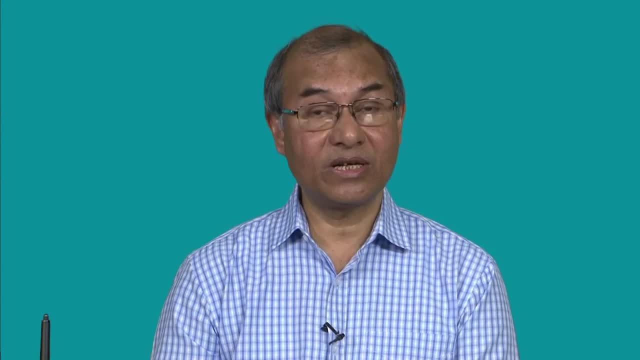 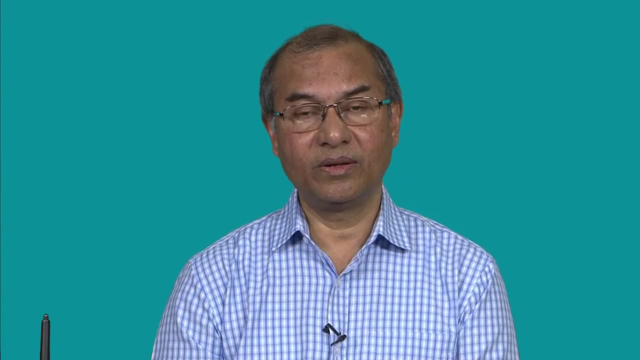 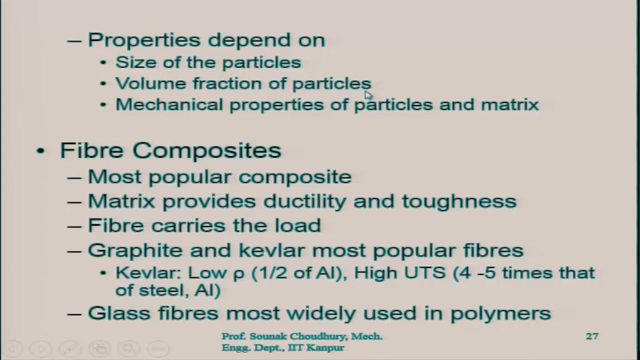 It will actually can withstand. it is better than in case of the particles which are larger in size, because the density is more and therefore it will be stronger, and so on. So volume fraction of particles has the same kind of an explanation why the properties can be better if the volume fraction of particles is more, but not in all cases. it depends. 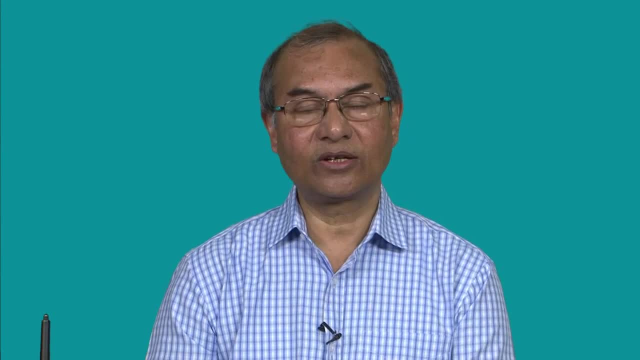 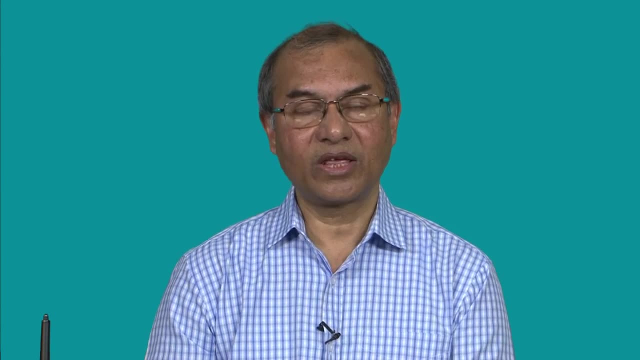 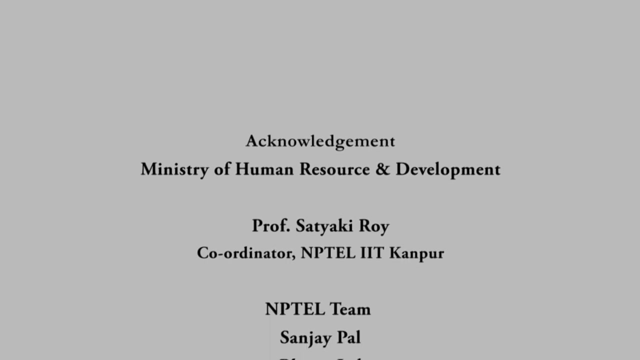 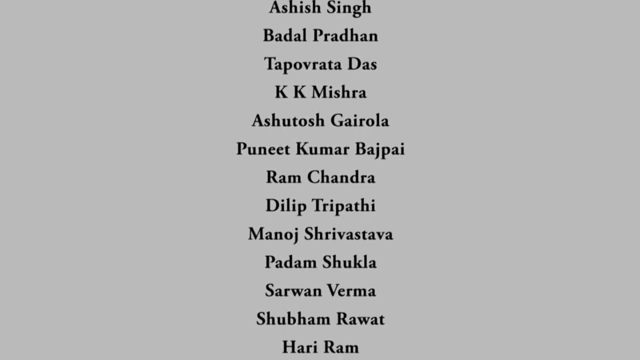 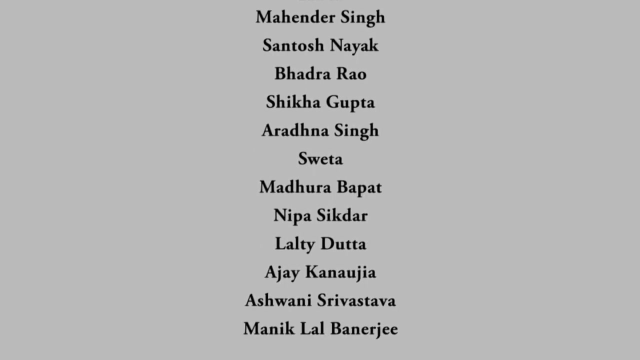 okay, So the rest of the things in the composite materials we will be discussing in our next discussion session. Thank you for your attention. Thank you very much.